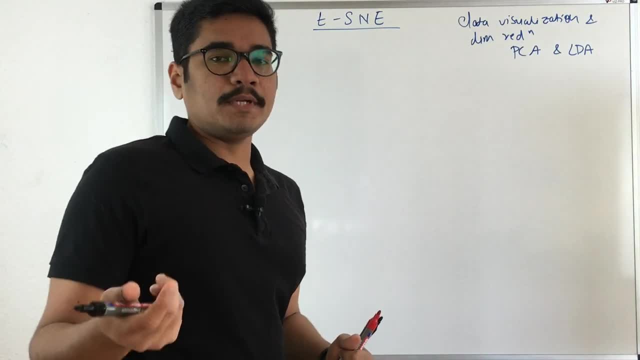 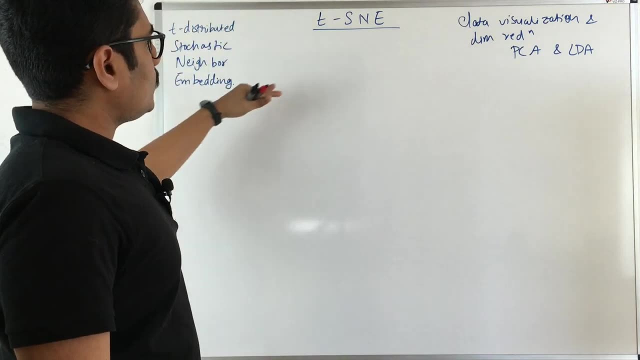 So that we mainly use in order to find the neighboring points, or which points are closer to each other, which are similar, And similarly we have Neighbor, and so it does the embedding of all these steps into one algorithm, Which gives us the package of T-SNE. 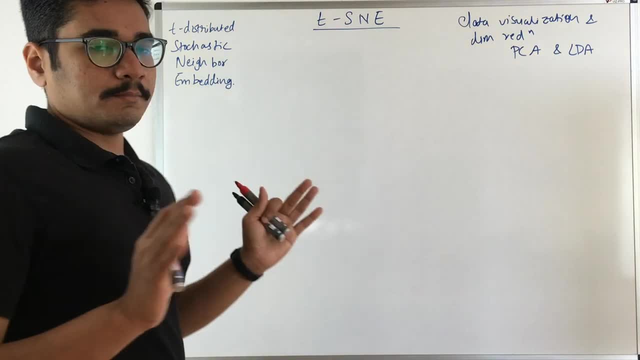 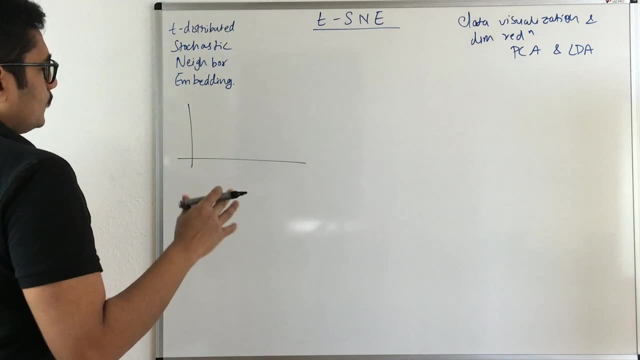 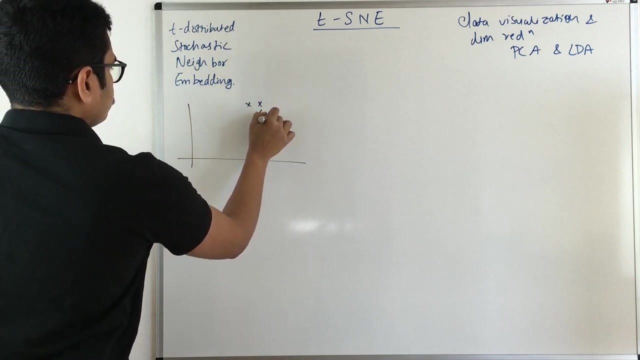 So let me give you a brief idea of what our major goal is. So say, for example: we have this dimension, So just we are for convenience, seeking for our two dimension. Now we have, say, some points. Say some points are like this: 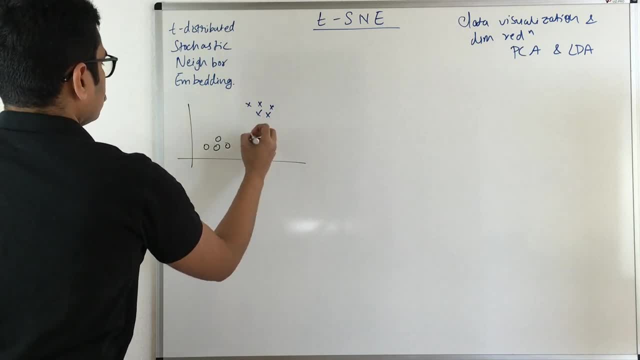 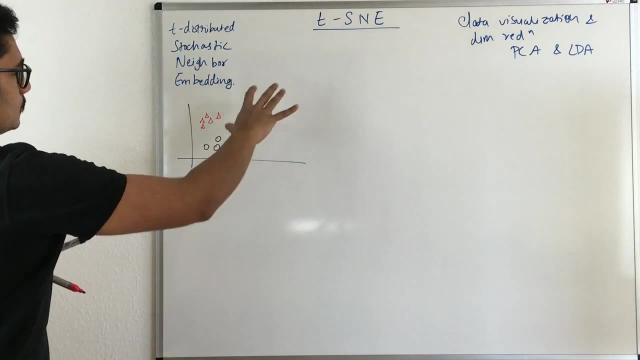 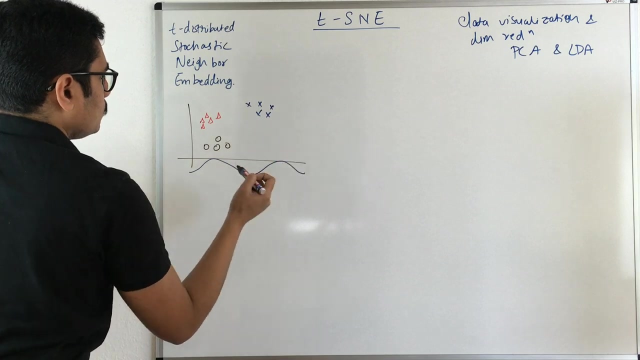 Some points are like this And say: some points are Like this. Now, if you see this, points are well separated or there are three different clusters that you can obtain. So usually if we draw a distribution, you get a distribution something like this: And you get: distribution for this, you get this way. distribution for this: you get this way. 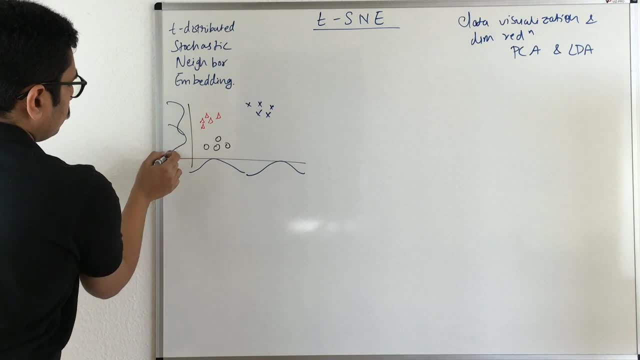 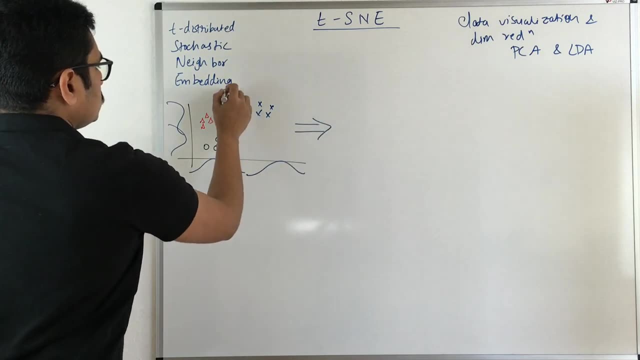 Similarly, you get one more distribution here and you have one more distribution here. Now what I want to do is Essentially convert this dimension. Now, this is in two dimension. Now I want to convert it into a one dimension. So how do I do that? 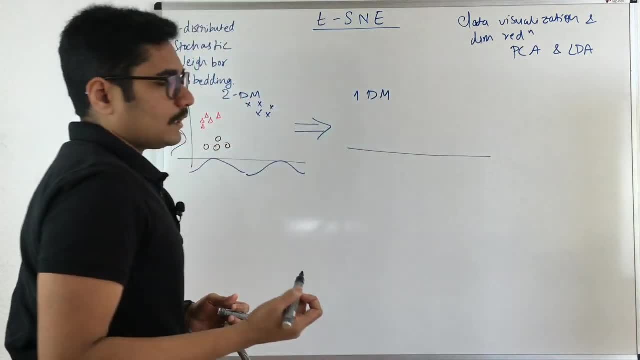 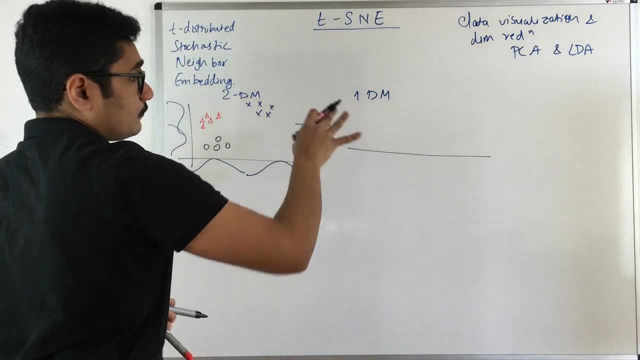 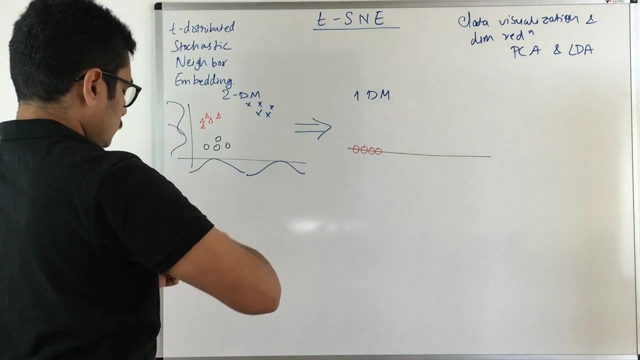 So basically just will consider a line like this: So a line is a separation, So you don't put all the points one above or below. since you have three different points, You have to cluster it accordingly. So We have some points like this: 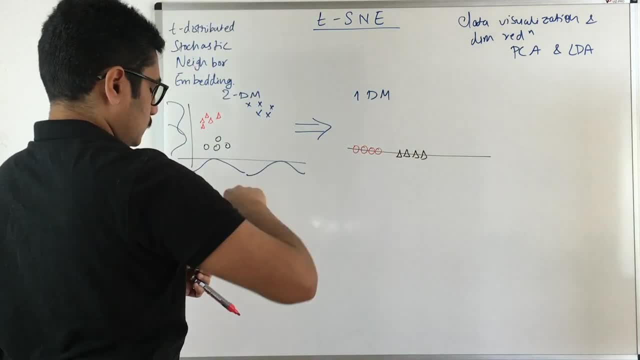 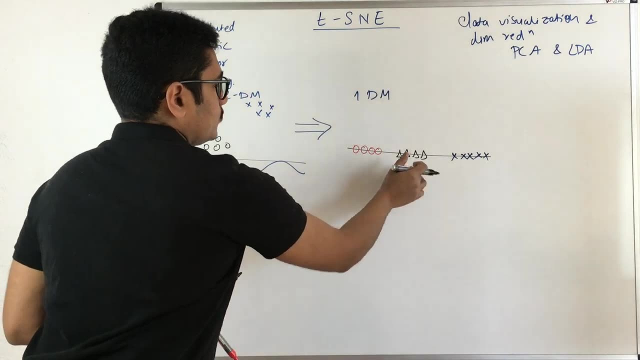 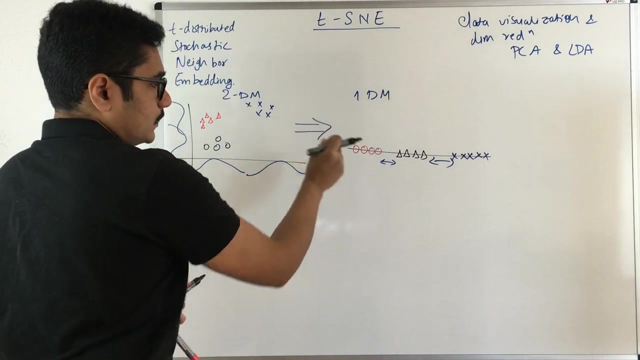 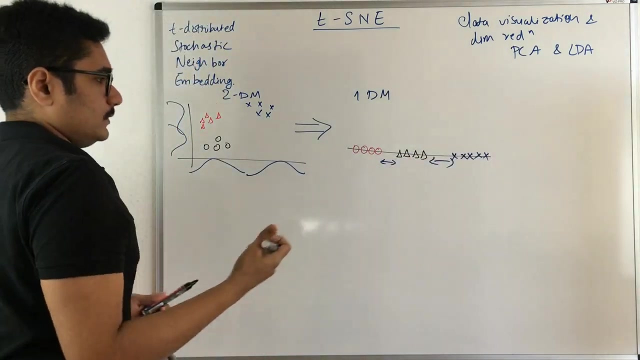 Then say Like this And say like this. So our major goal is to have a separation of these two points From each other in this way, in this approach. That means similar things are similar. objects or samples should come together And there should be some gap or some separation from the other samples. 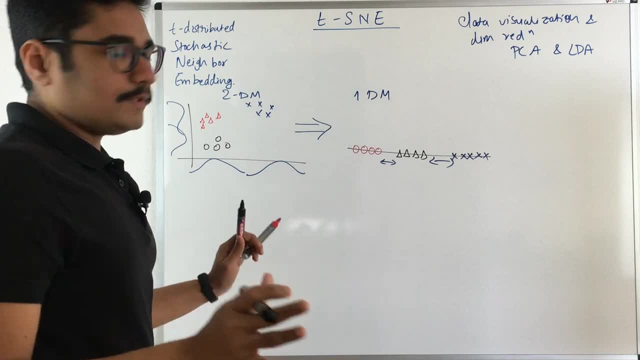 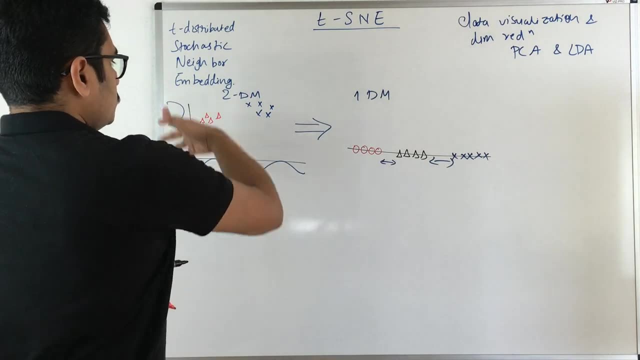 So this is our objective, But usually in the real world you don't get the points in well separated or in In a very neat manner. So what do you essentially get? is you get a mixture of all these points. So you can see essentially in this example: 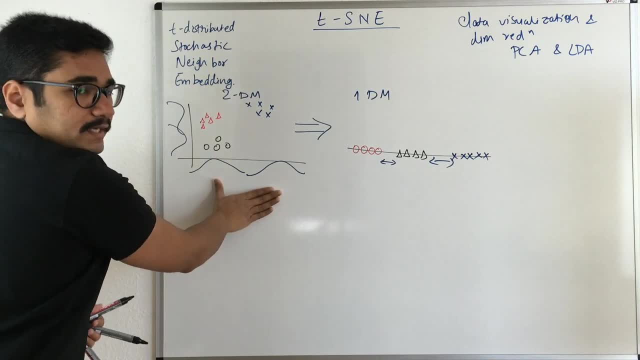 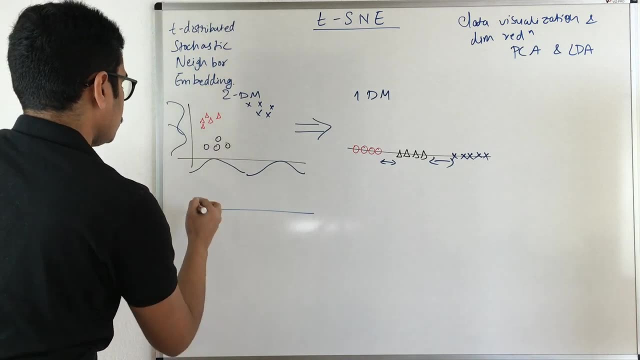 If you project all these points onto the x-axis, that is, on this one, You get the distribution like say: here: in this case You have all the crosses, So That's not a problem. But when we project these two points Now, you can see the graphs of these two are overlapping. 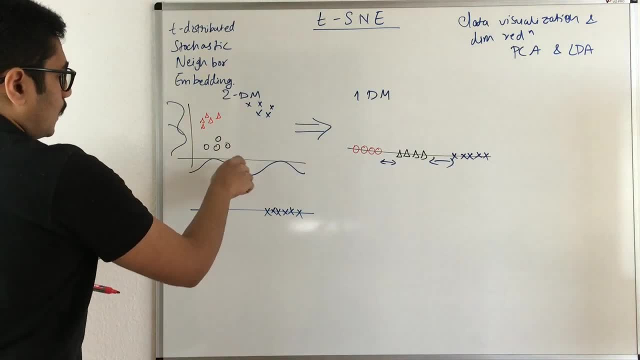 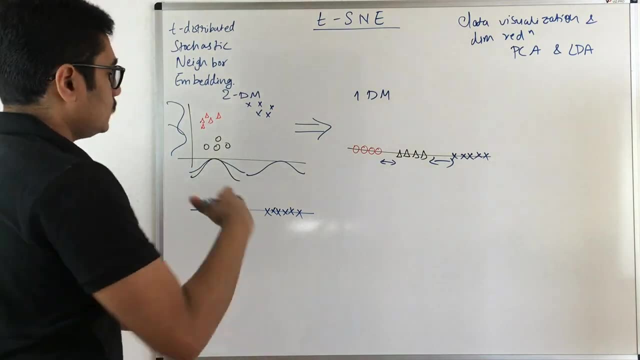 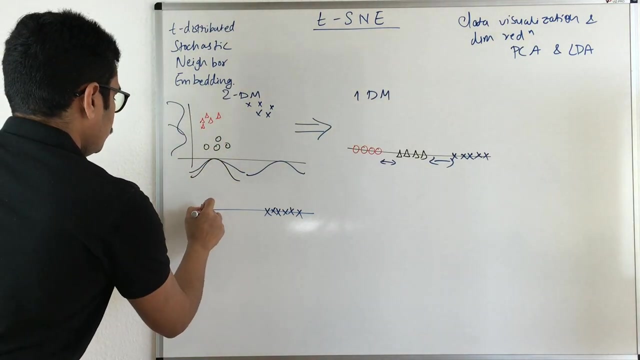 So whenever you do a visualization, you get a graph which is more or less overlapping, So you can't make out like how many different points or distinct two clusters are present in the original data set. So this is our original dimension. So here, as a result, we get the output as: 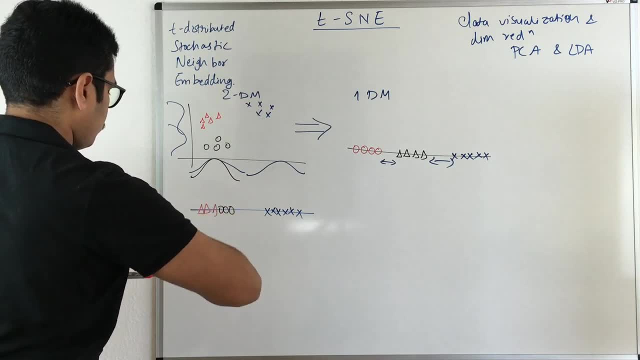 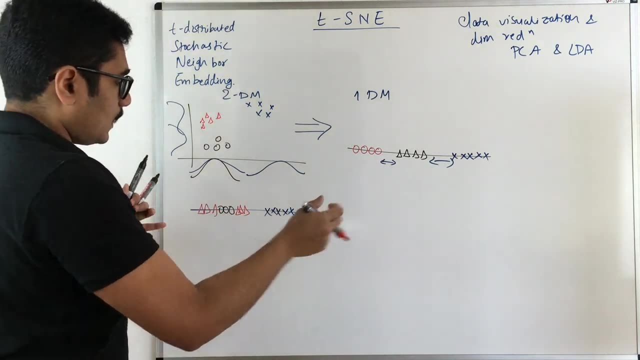 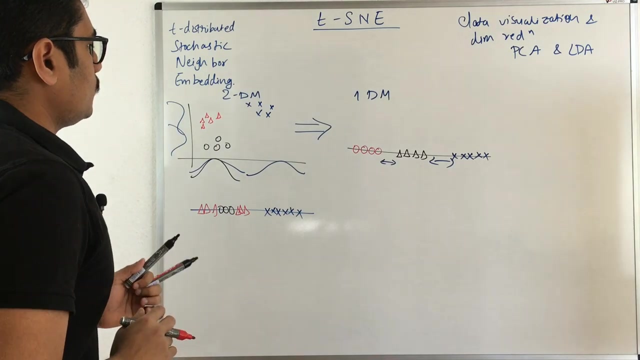 Say some points are this way And like this Or in any manner. So assume like this is a stick and there are different beads, So you want to arrange this beads into different categories. Now how would you do this? So basically, we use a technique called as SNI, that is, stochastic, neighbor embedding. 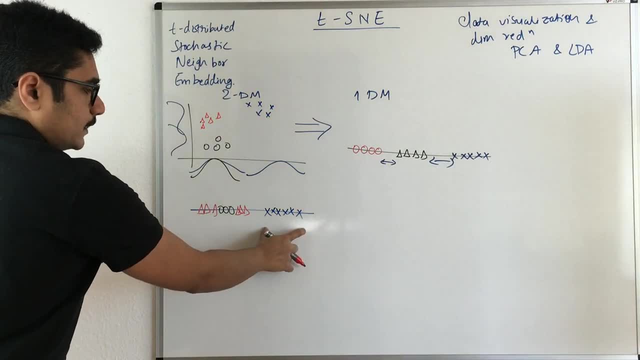 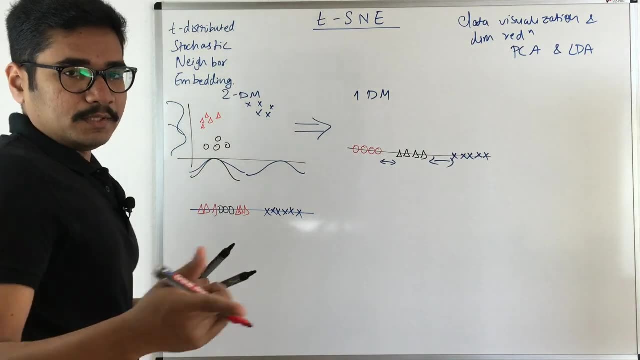 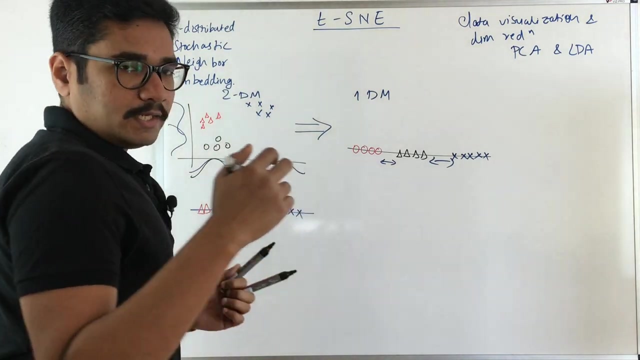 So we have some error in this. But this particular sample or this particular category is pure. But here we have to do some techniques so that we can just minimize this or we can just separate it out. So how would you do that? So essentially for this, what we do is we take a normal distribution. 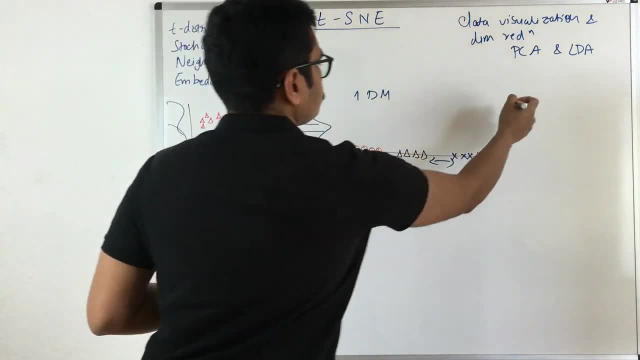 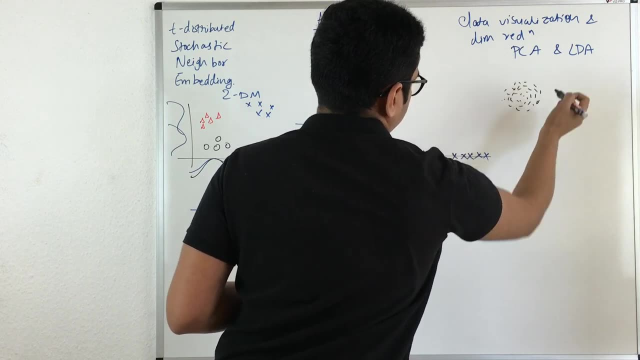 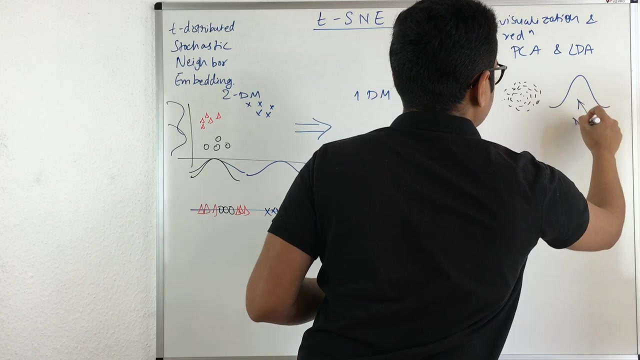 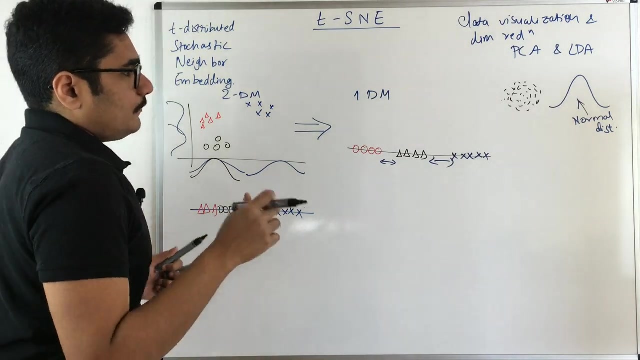 So whenever any points are there. So we already know that if there is a distribution of points, say, which are globular or which are spherical in shape, As an end result we get the distribution something like this: So this is your normal distribution. So what we have is: 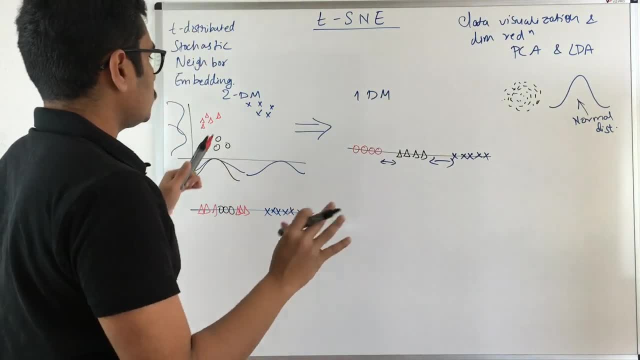 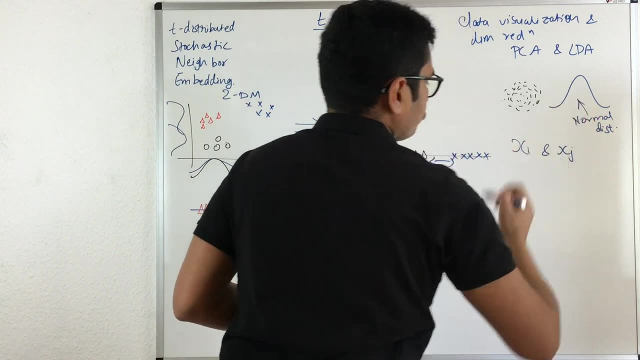 We take a joint probability. Now say, for example, in this case we have so many points, We are just considering only two different points, That is, xi and xj. So if we want to find, that is, whether xj is a neighbor of xi or not, 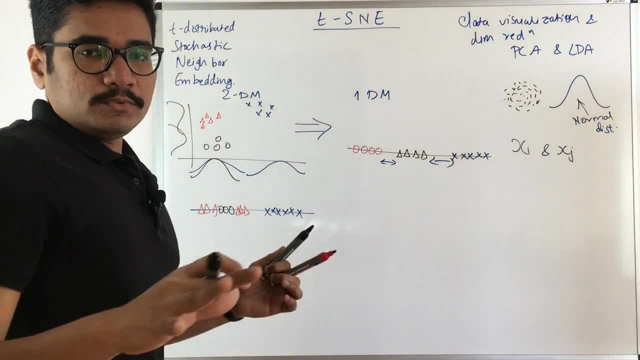 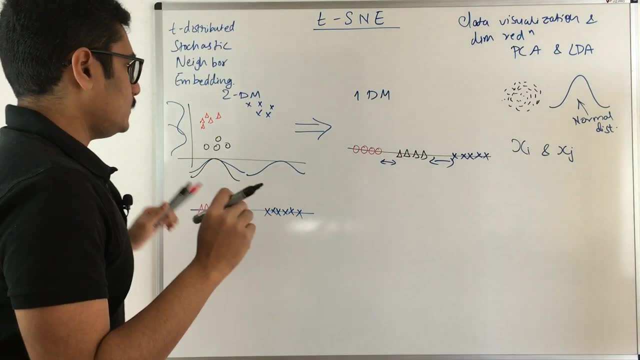 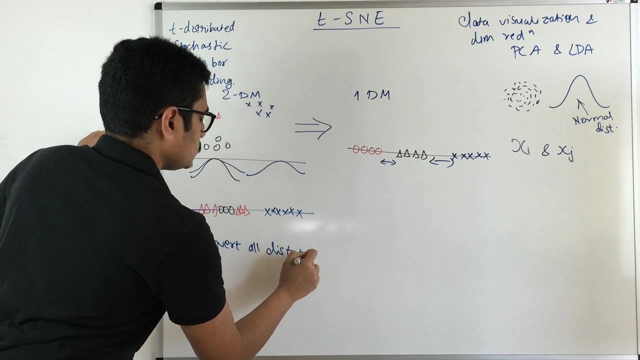 We want to just estimate. So basically, what we do is we convert all the distances which are there in this particular matrix into probabilities. So that is the very first step that we do, That is, convert all distances to probability values. How will you do that? 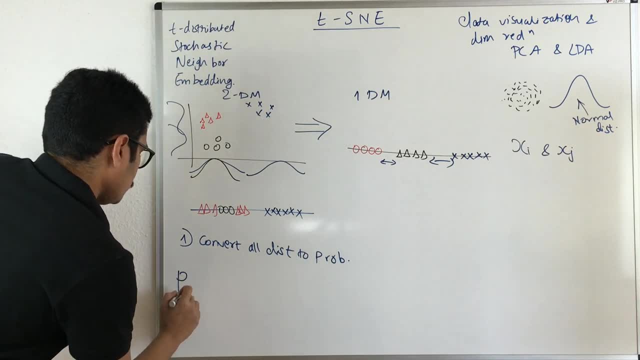 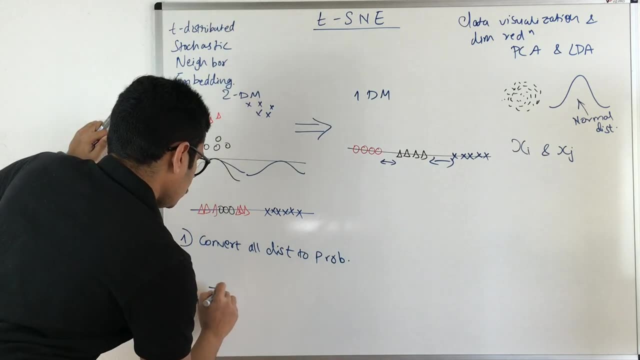 Say you have a probability, say P given for point j, given that xi is there. So how would you estimate this? That is e raised to minus xi, minus xj, square upon 2 sigma i square. Now this particular value is a very large value. 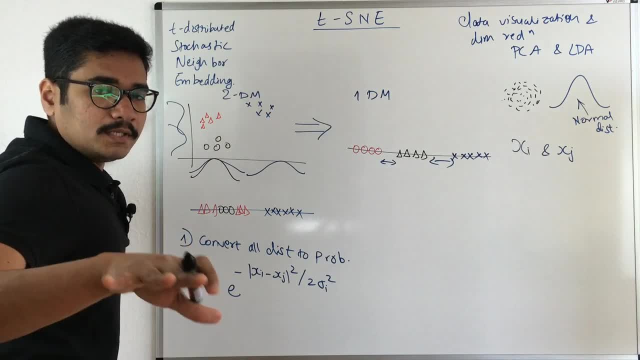 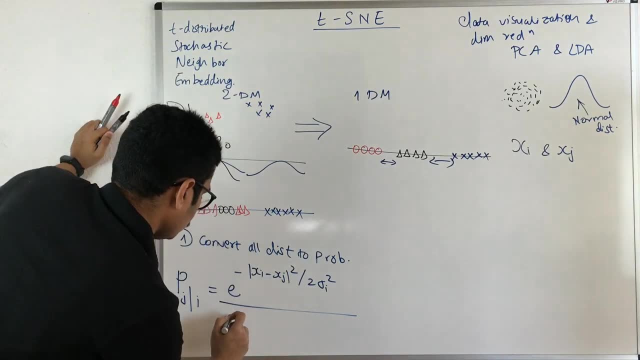 So, since probability values cannot be large, It has to be minimized to 1 or within that range. What we do is we take a submission of all, we do the normalization of all this. So which is e raised to minus xi minus xk? 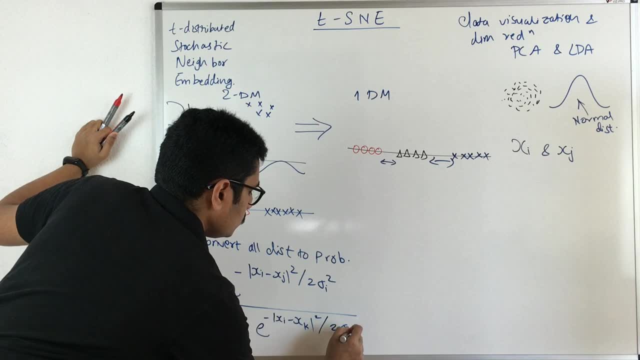 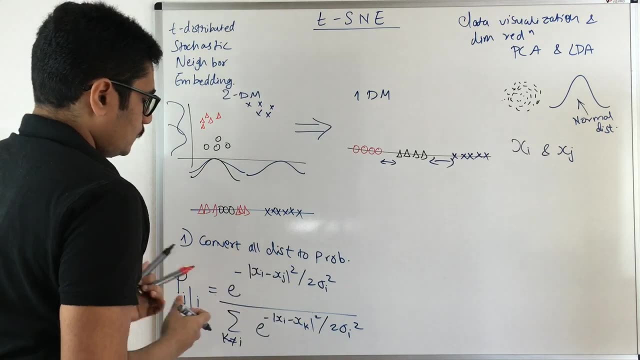 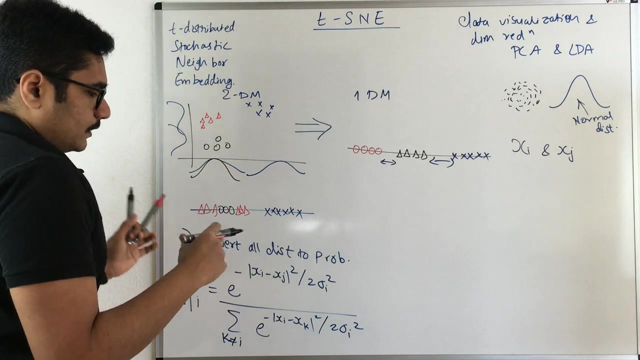 Say, we have k number of points upon 2 sigma, i square and k not equal to i. So this is the formula we follow for normal distribution if we have the points in this way. So if you look at this, you are familiar with more or less the terms. 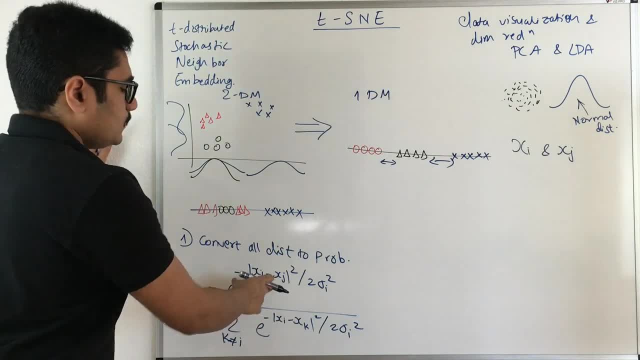 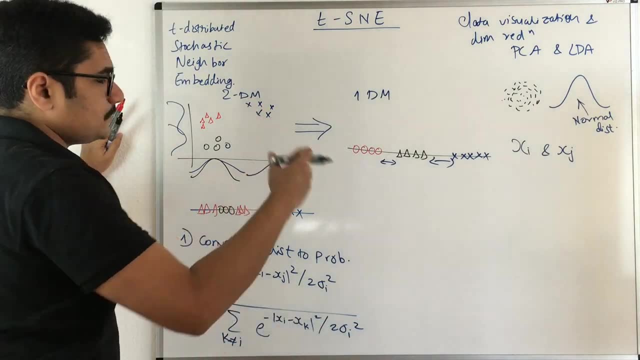 So this is nothing but we have already seen in many videos- is nothing but our error. So here we don't calculate the mean. instead we go with the variance of how the distribution or how the points are. But if you remember, for the formula for normal distribution, 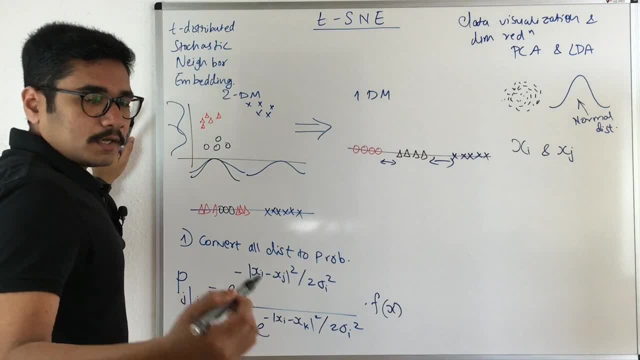 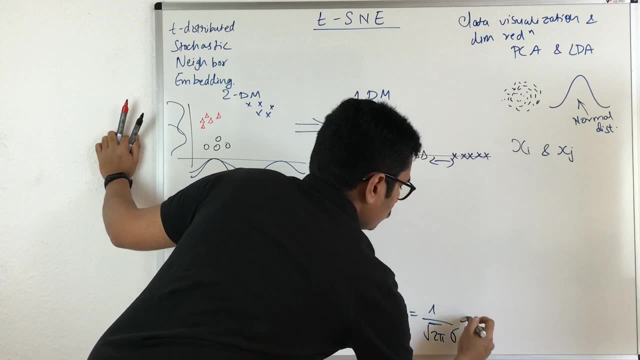 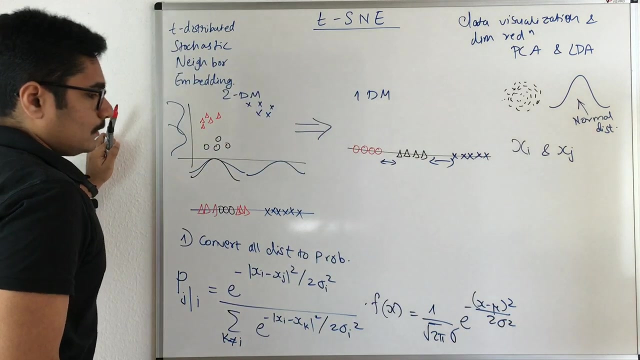 Say: we have a point, Say x, and if you are about to find the normal distribution of this, how would we do this one upon root 2 pi? Then we have Sigma e raised to minus x, minus mu, the whole square upon 2 Sigma square. 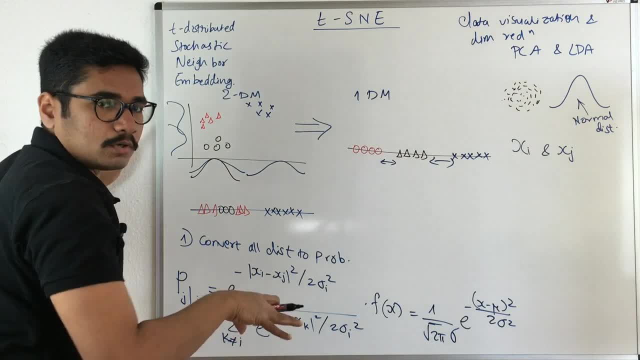 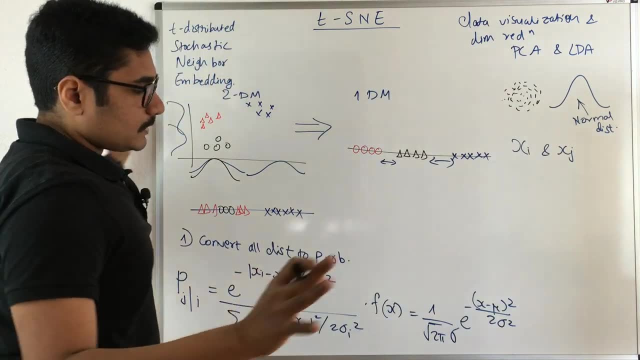 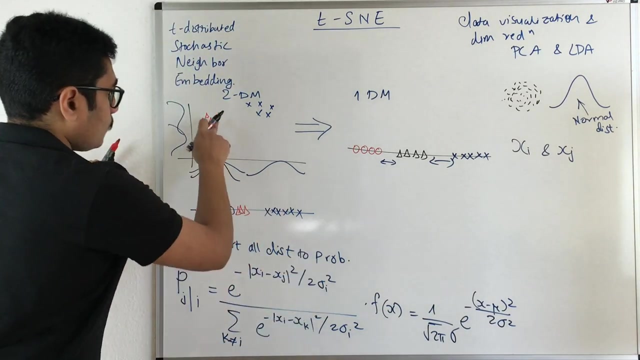 So if you compare this formula with this formula, it's more or less same. But here, if you see, you have a variance that is a global variance. So the variance across all the points remains constant In all the spaces. But here, when we go with each and every point, 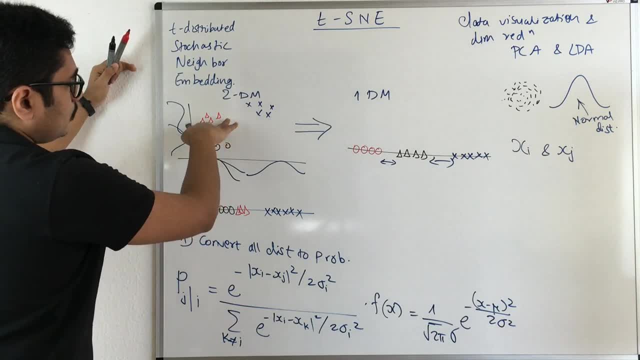 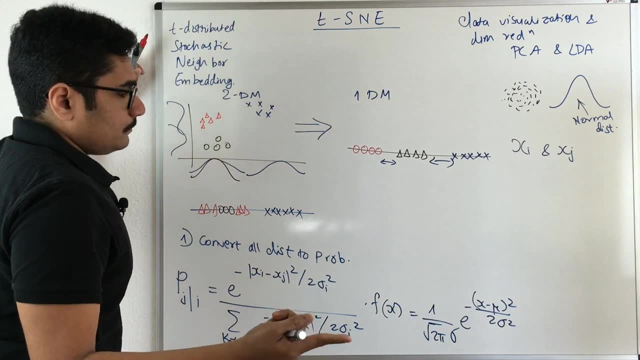 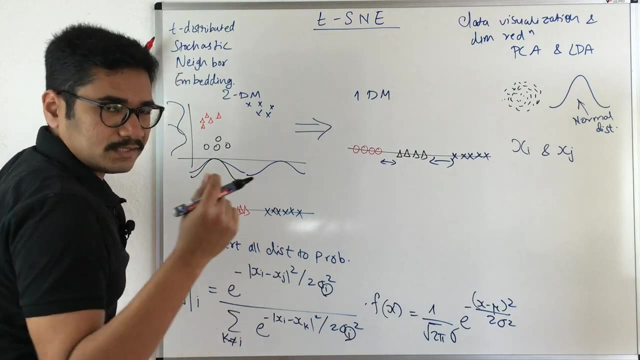 So you can see the distribution of points in, or the variance of points in, this distribution or in this cluster, on this cluster, all are different, So we essentially want to get rid of this. I, that is the iteration which is taking for each and every point. 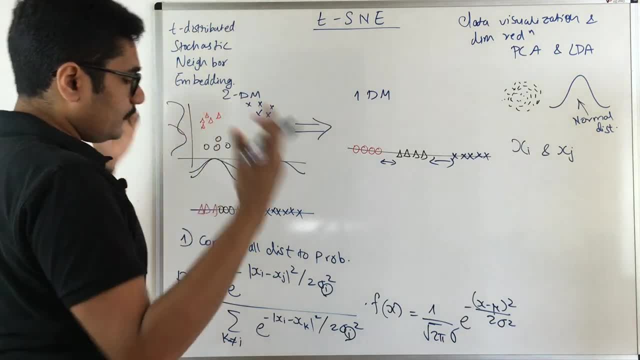 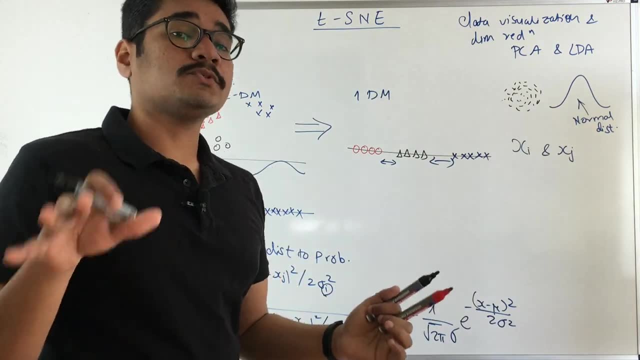 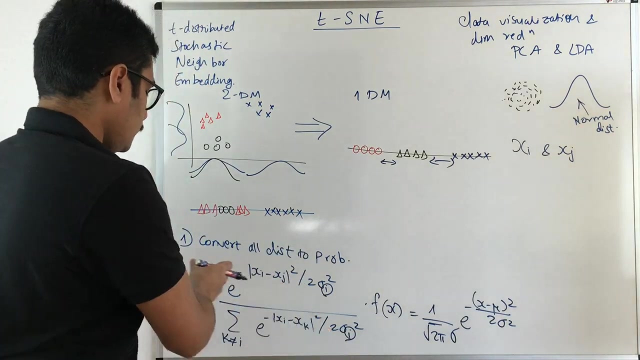 So, with different variation of different data points and different spaces, We cannot hold this formula and keep it for so long. So since this is used for visualization, we can't take this also there. So essentially, we want to get rid of this. So what we do is we project this probability points or we just reduce the dimension to some other space. 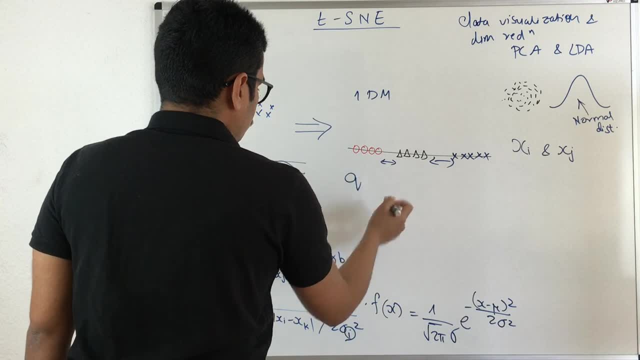 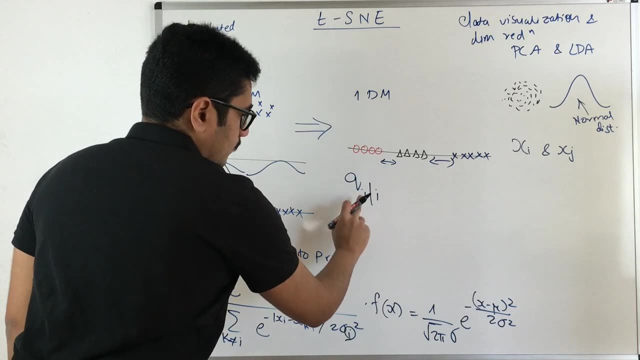 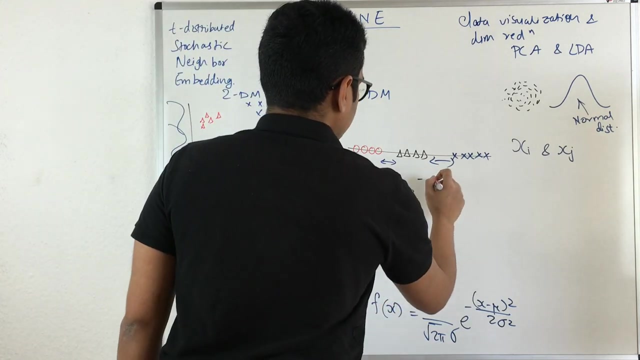 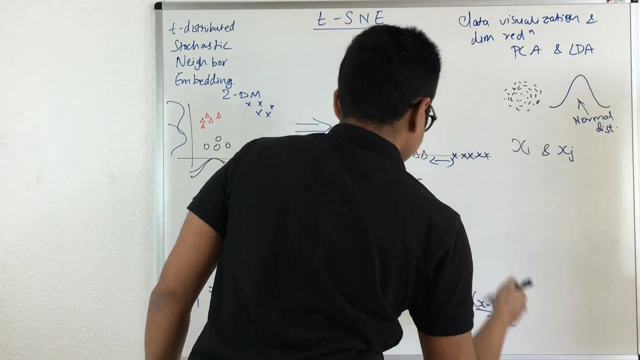 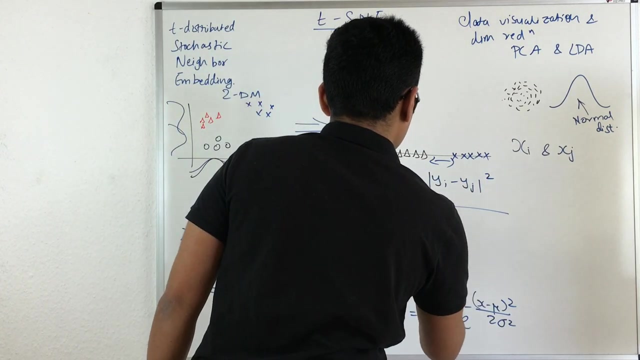 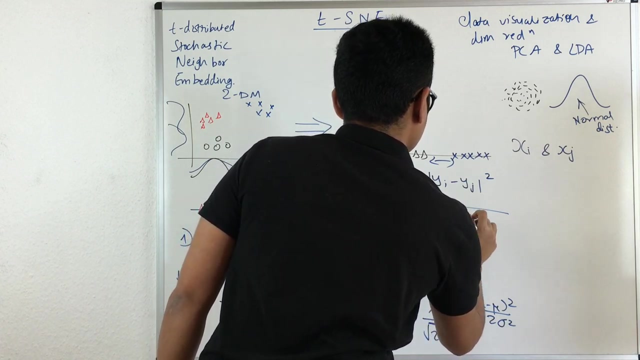 So say that other spaces represented by Q and say we are estimating the values or the neighbors for point J, given You have a point I. so how do we write this? So this formula just becomes X- I minus. here. instead We just change the representation to yi minus yj. square upon K not equal to I e raised to minus yi minus yj. 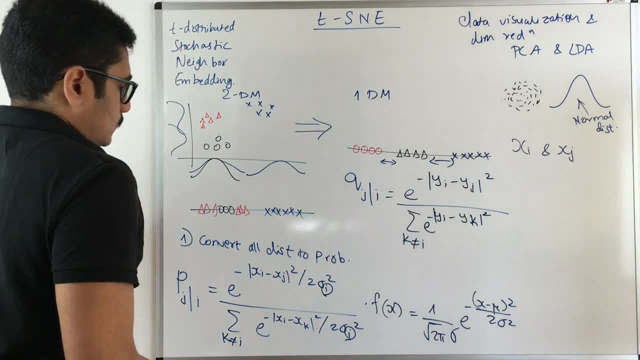 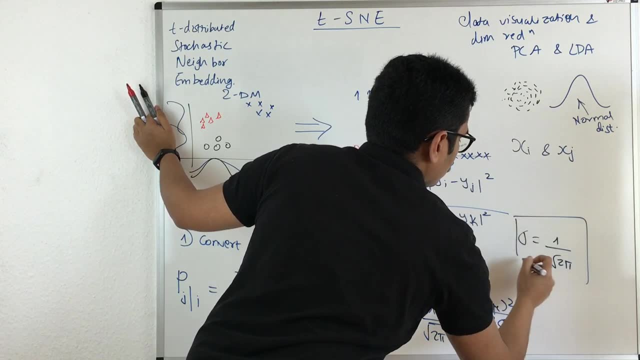 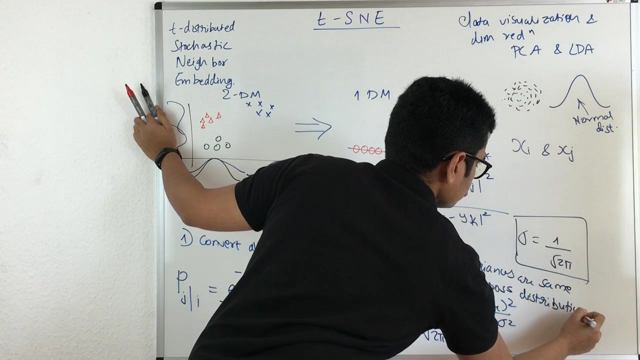 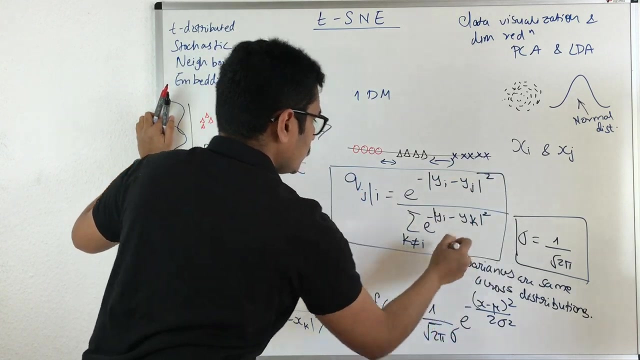 yk Square. So here we can assume that Sigma, that is, standard deviation, can be 1 upon root, 2 pi, And we are assuming that all variances are same across distributions. So this is the dimensional reduction part, what we have done. 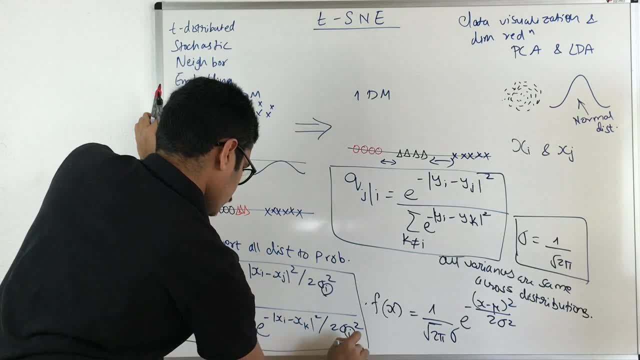 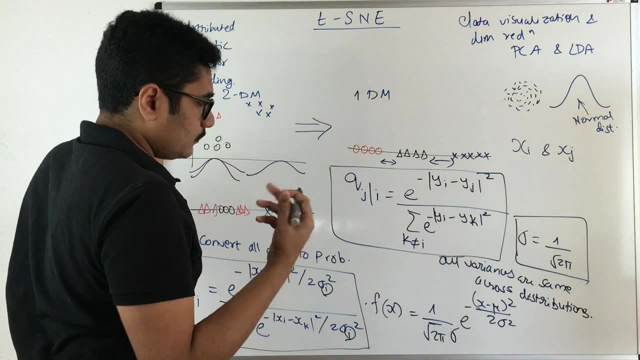 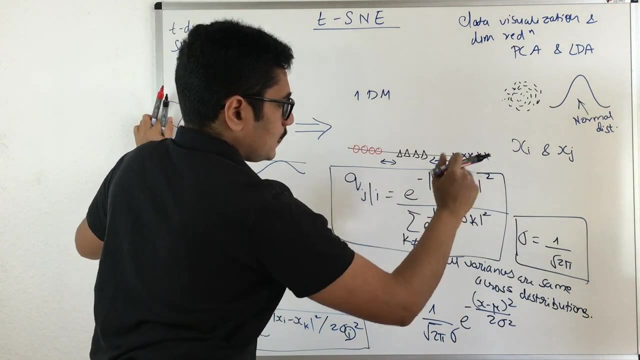 So this is what our original formula is. So in the higher dimensions, since we had a variation in each and every data point, we cannot take that for our calculation. So instead, what we did is we just projected all those points into a dimension Q and we have just kept the variance across all the distributions, or all the spaces, as same. 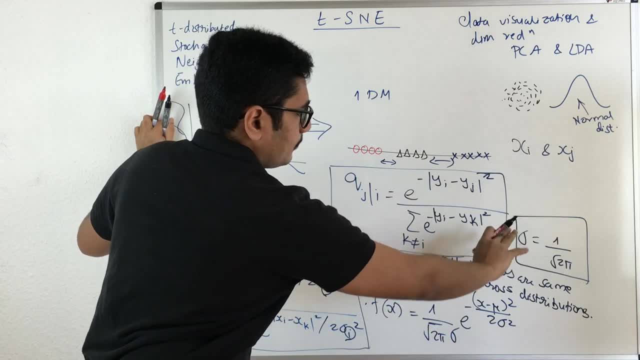 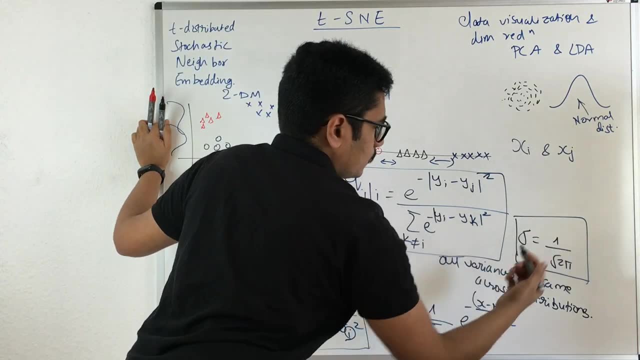 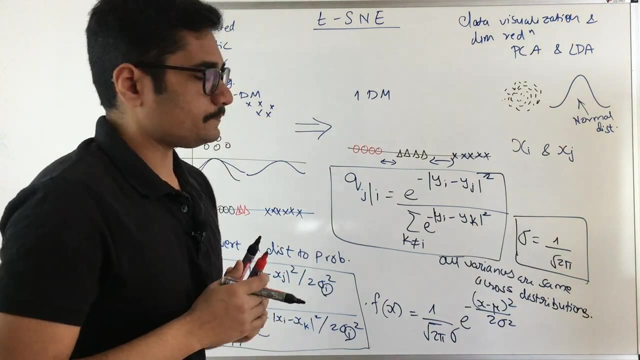 So we have just eliminated, Or instead we have just kept aside the Sigma, or that is the variance term. If you just square this, you get the value that is 1 upon 2 pi. So now, how do we measure the distances between two of these points? 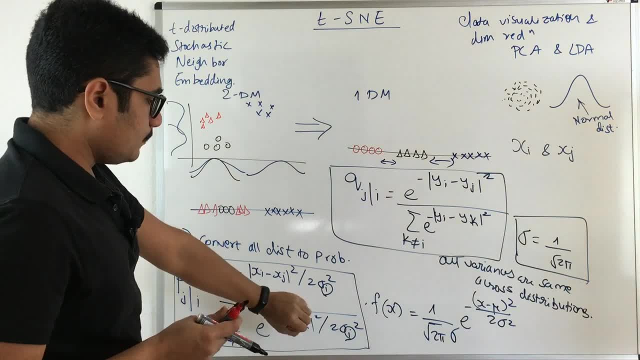 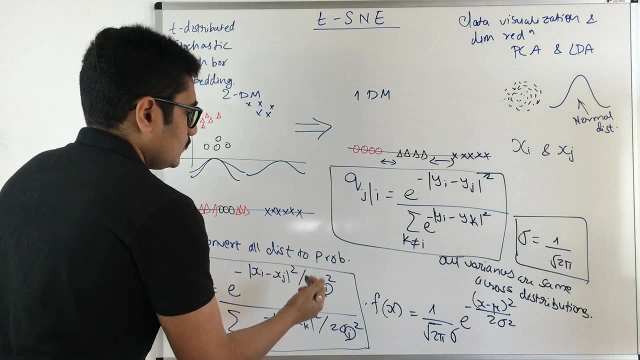 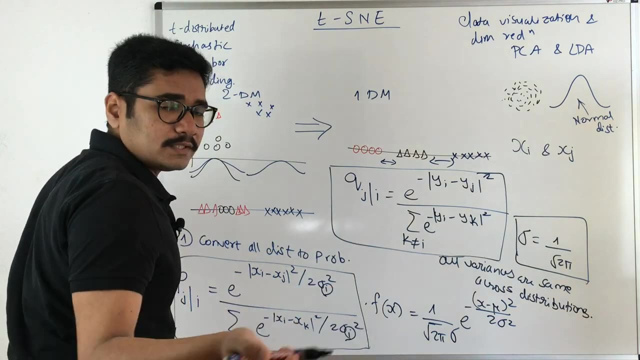 So, essentially, when we removed this Sigma I or instead the Sigma term from this, what we essentially had is here, in this case, when the points were like this, Or when you had the symmetric, or when it was symmetricity, or when there was a symmetricity across all the points. 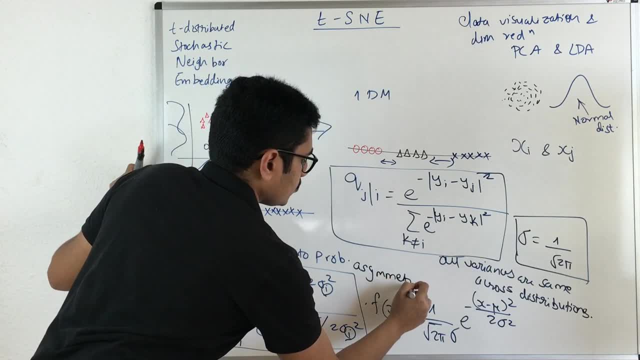 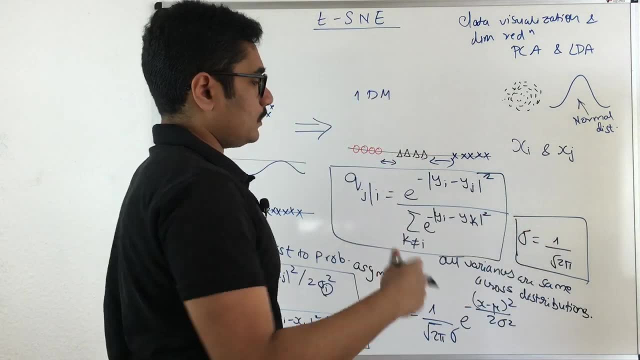 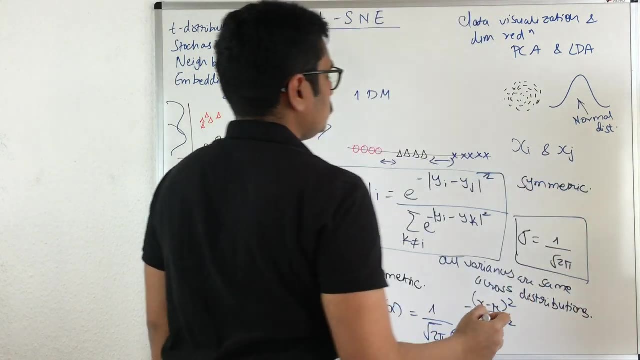 It was asymmetric distribution or the points were more or less asymmetric. Since you have now one standard deviation or the variance across all the points, you made it symmetric. So essentially, one main step when you do t-SNE is that you have to make the distribution as symmetric. 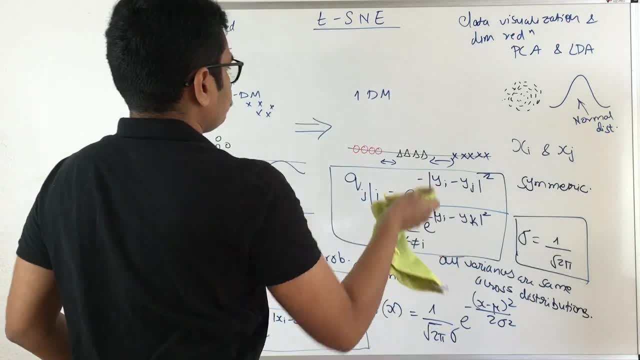 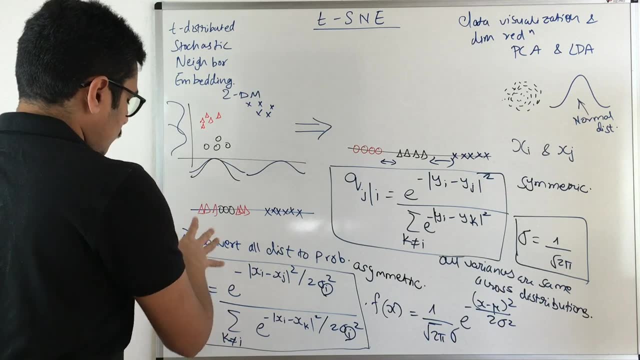 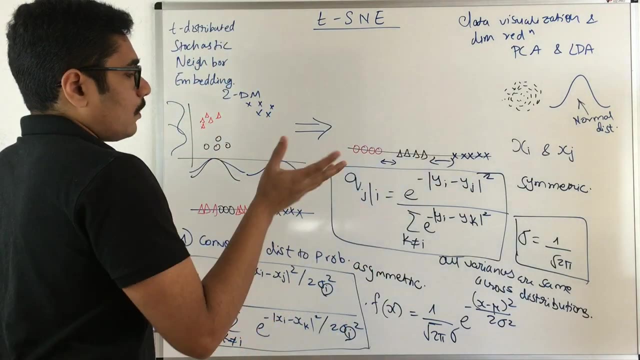 So that is the first step, The first point you have to keep in mind. Now, what we have done is we have this representation in some higher dimension of this and we have projected into lower dimension by making it symmetric. Now, how do we measure the distance between the two distributions? 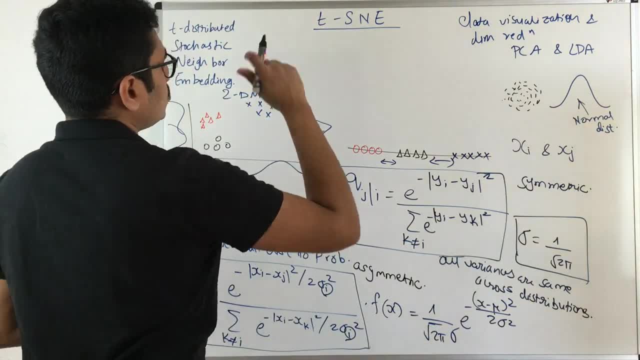 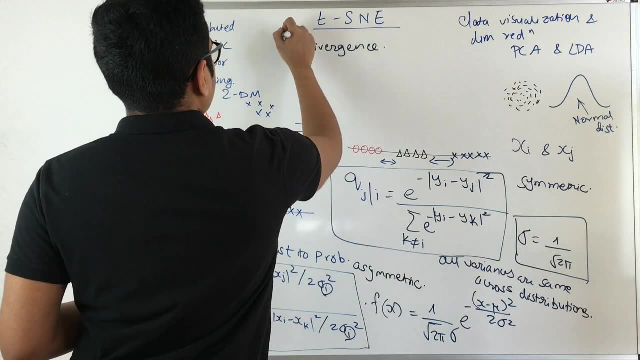 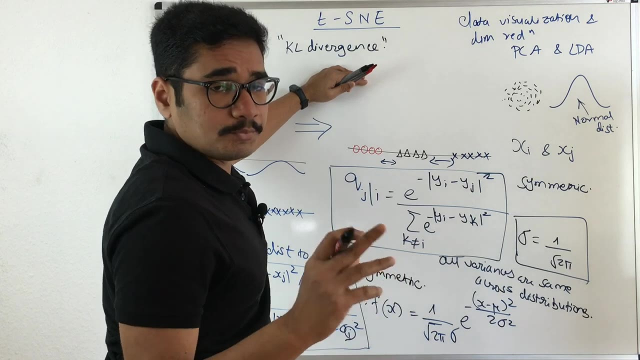 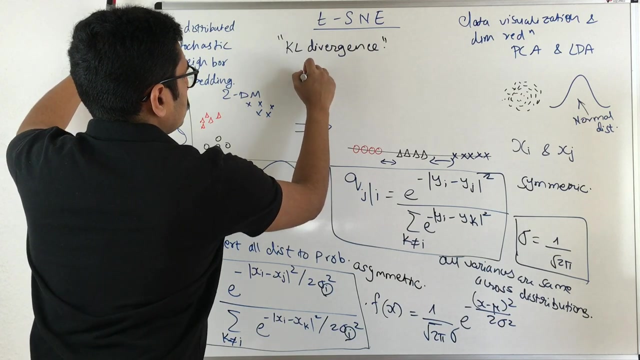 So essentially what we have is we have a distribution measure called as KL divergence. So we mainly use this particular divergence technique in order to find the variation or the distribution among the distances in the data points. So essentially say we have P, Q, So KL divergence of these two. 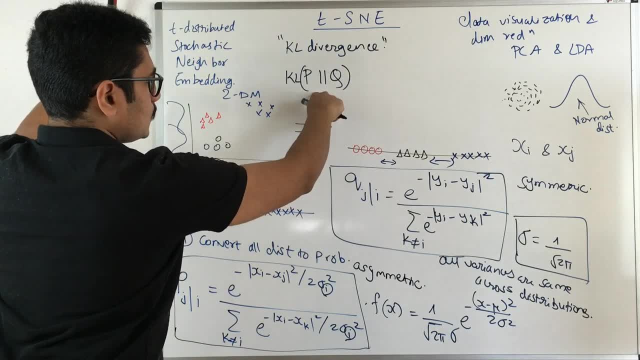 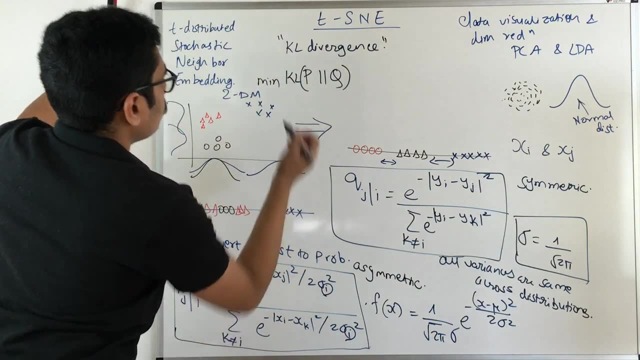 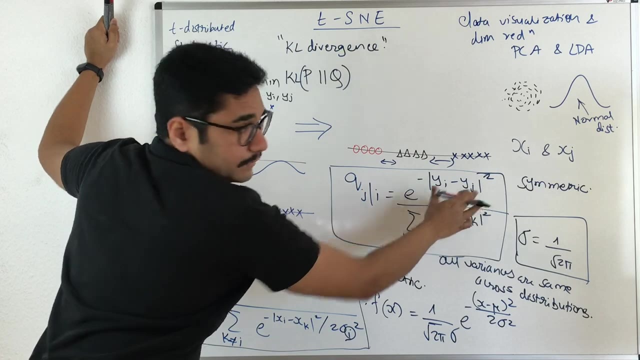 So it's written in this way. that is a KL divergence of these two dimensions. So P and Q represents two different dimensions and we want to minimize. What we have is yi and yj, So now our points will be yi and yj. 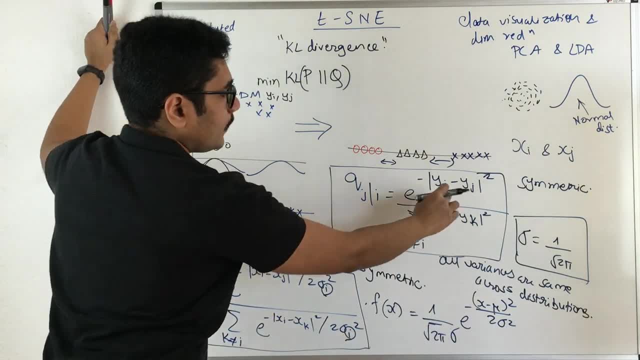 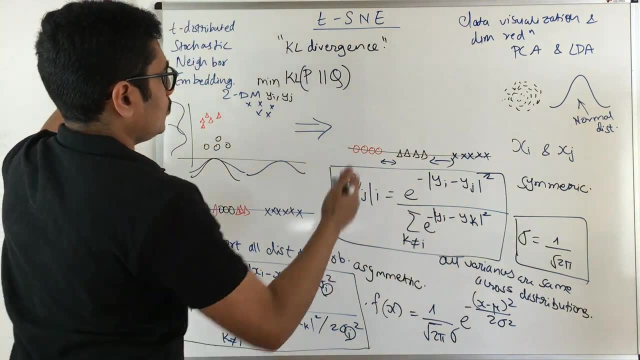 We have converted from xi and xj to y and yj, So now we have these points. So now we want to change this particular equation, or how do we achieve that? So this is given with respect to the first dimension, that is, the original dimension. 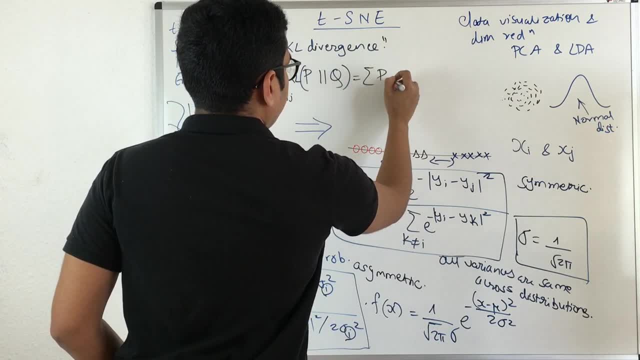 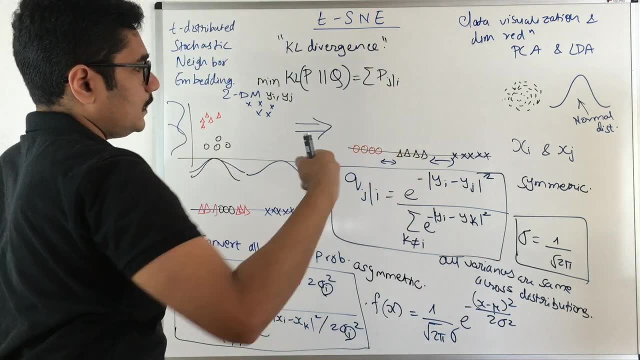 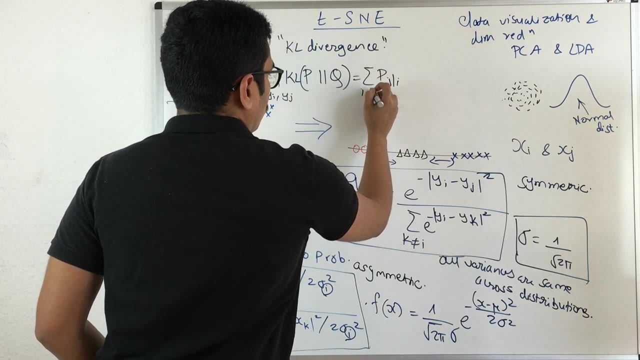 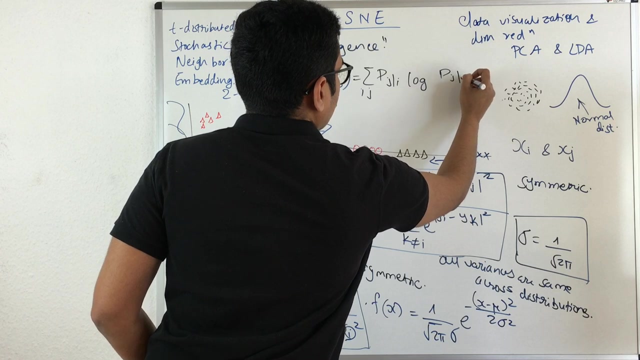 So we take that is summation over P, J given I. so this is basically conditional probability. But whenever we calculate the distribution across the two deviations or the two dimensions, we mainly use a joint probability. So it becomes ij. Then you take the log of this: PJ given I upon QJ given I. 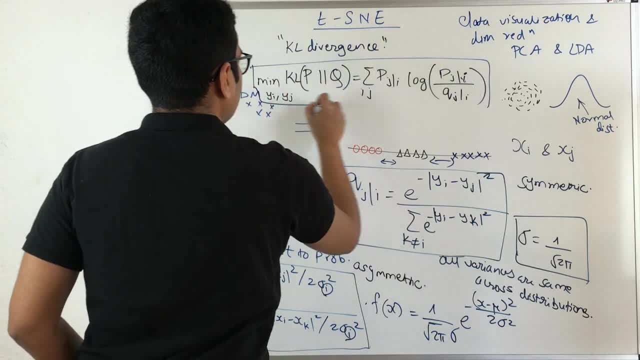 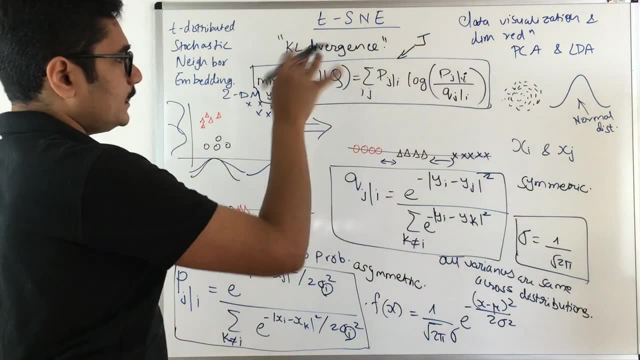 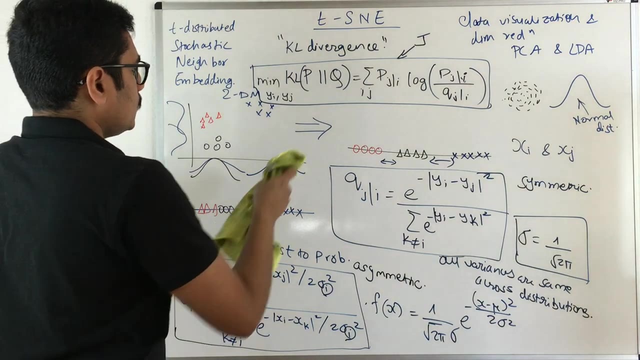 So this is your function, which you need to minimize. So, essentially, this is nothing but your J, that is your cost. So then, further, what we do is we take the derivative of this, then we do the gradient descent and then we calculate the minimum. So obviously, from this equations, there are two things to be drawn as conclusion. 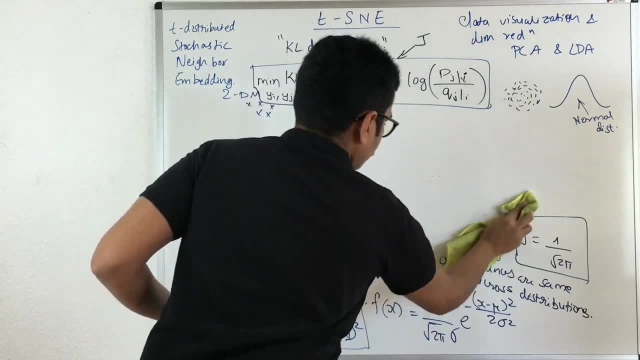 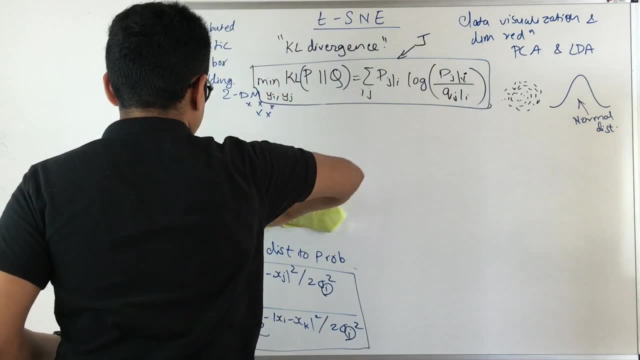 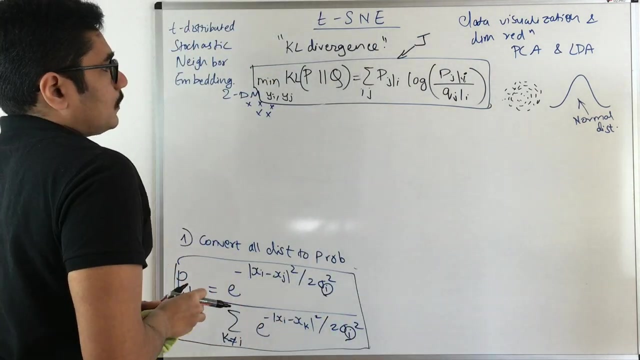 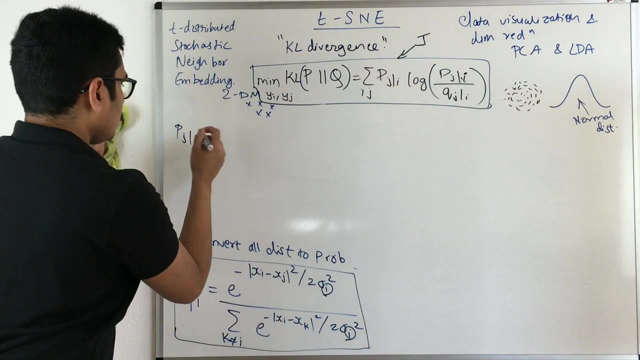 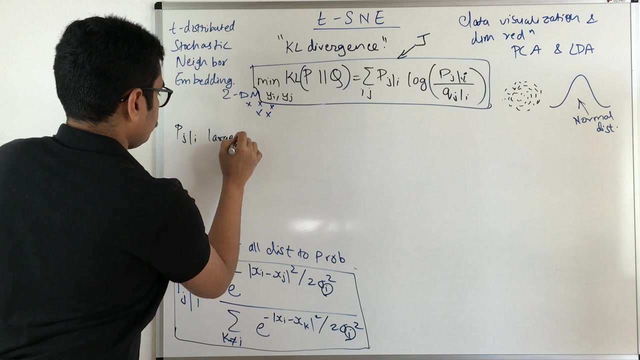 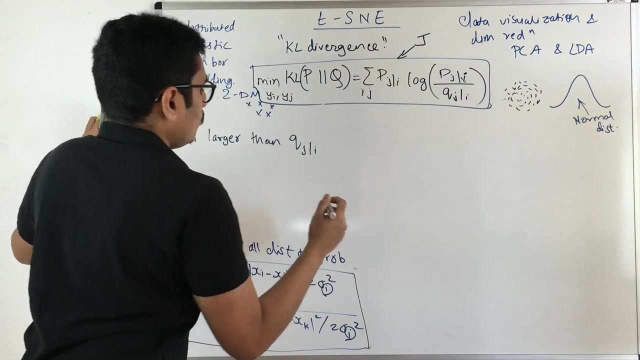 So So now, since you have this log ratio, So if you have PJ I, that is, if your probability value in the original dimension is modeled, or if this is larger Then QJ given I, Then what you incur is the log of a large value. say, for example, in this you have two and this you have one. 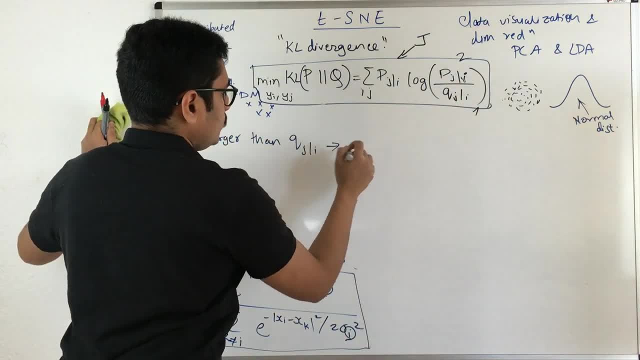 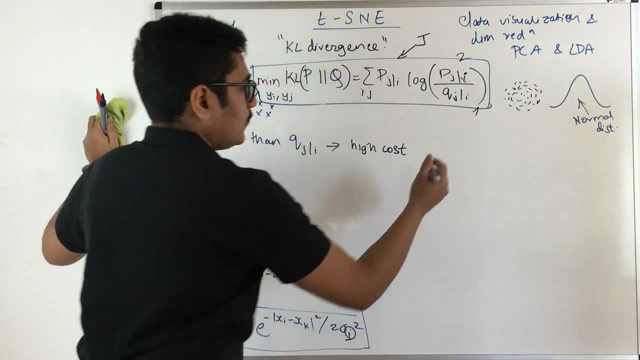 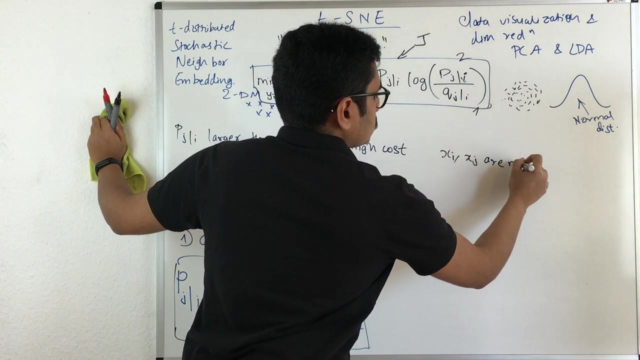 So log of a large value is large, So you incur a high cost, But you need to minimize this. So what this essentially says is that XI and XJ, which are representative of the original dimension, These two are neighbors But in the 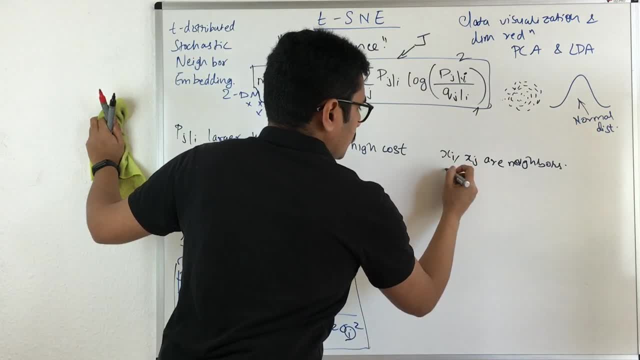 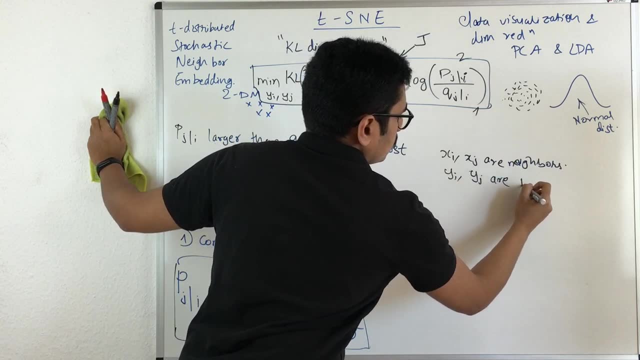 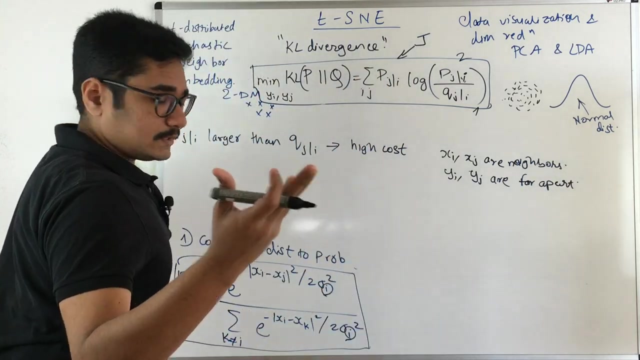 But in the lower representation or in the reduced dimension If it is YI and YJ. these two are far apart. So we don't want this. That's why we have just changed the variance term and we have represented in some other form. 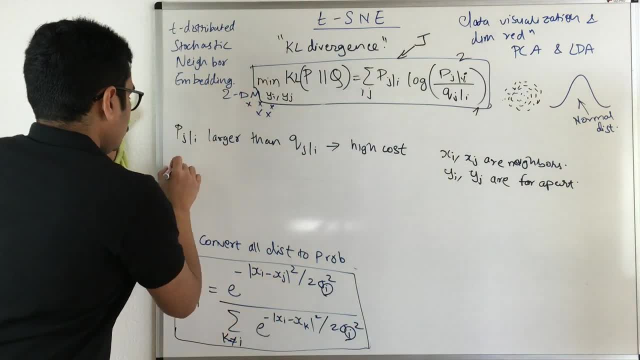 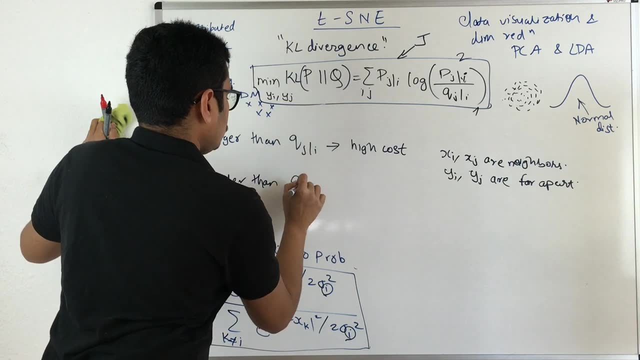 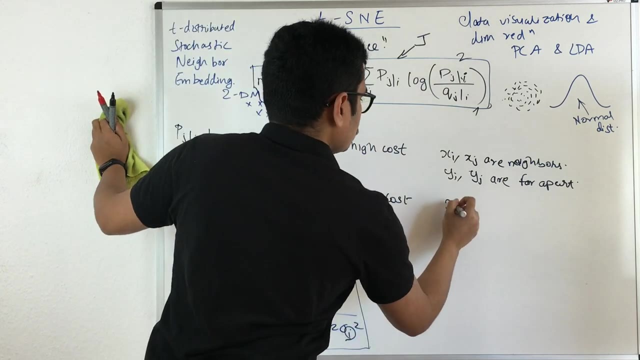 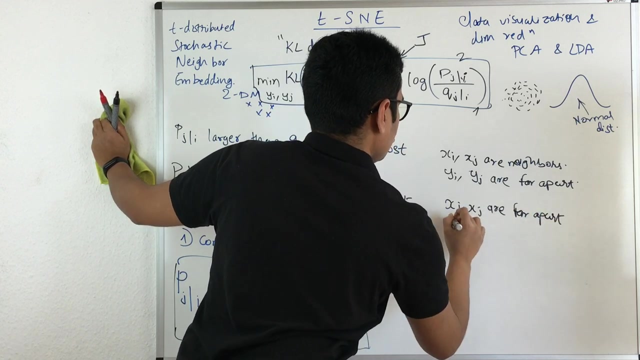 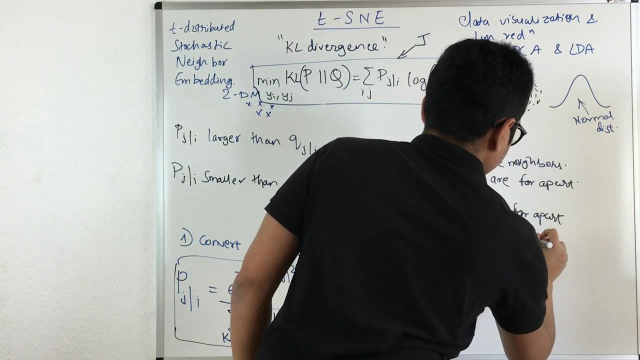 So we want our equation to be in that form: And if your PJ- I value- is smaller Then QJ given I, then it incurs a lower cost. That means XI and XJ are far apart. That is in the original dimension, and YI and YJ in the new reduced dimension are the neighbors. 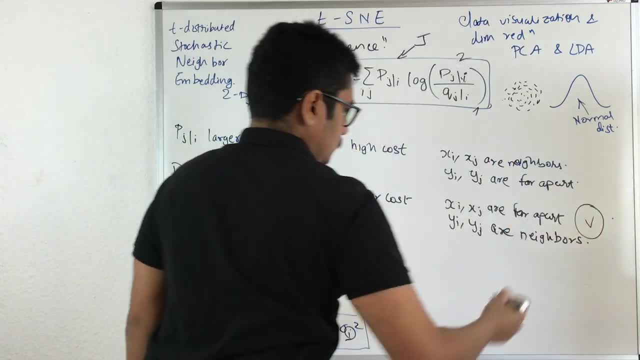 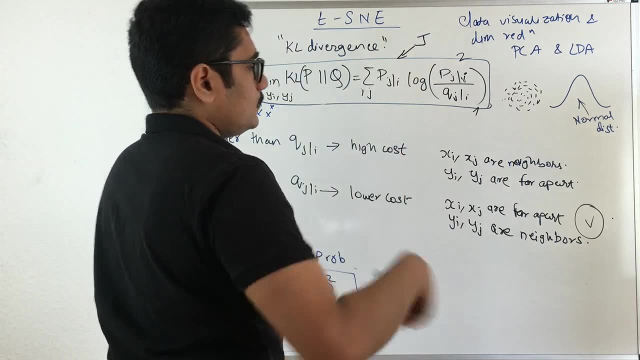 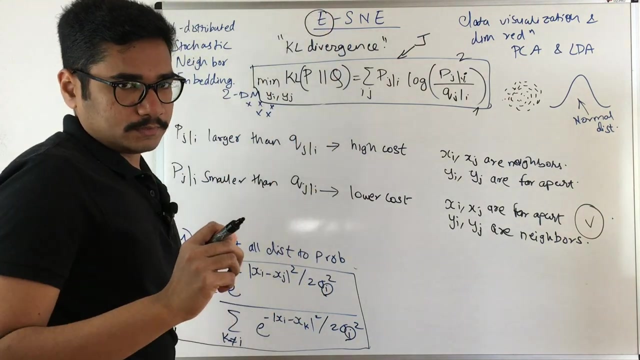 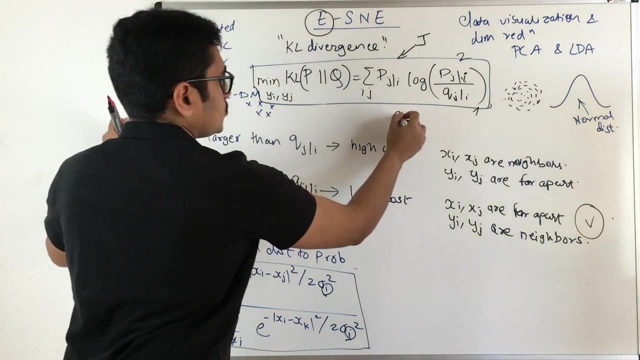 So this is what we want to achieve in this. So, essentially, we go with this particular approach. Now, this was all about SNI. Now, what we have is this T distribution. So what is the main purpose of this T distribution? Now, the modified formula with the help of T distribution on your Q dimension, that is, earlier it was QJ given. I. 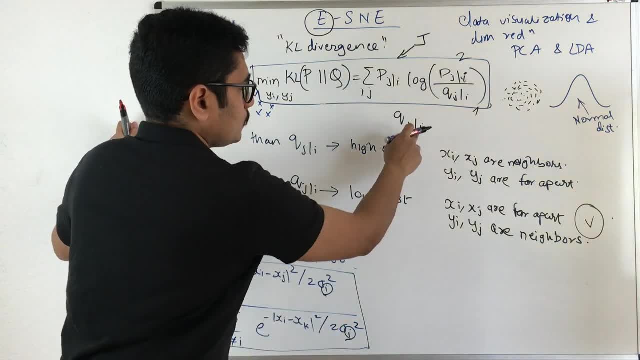 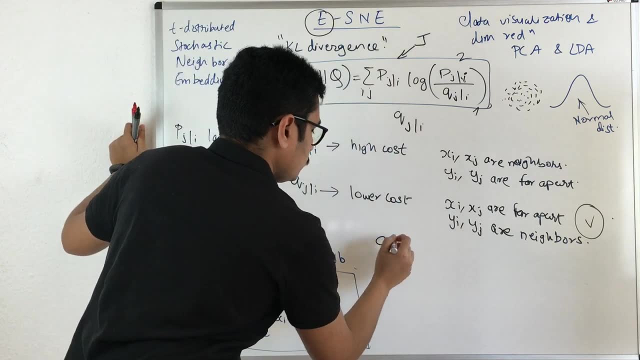 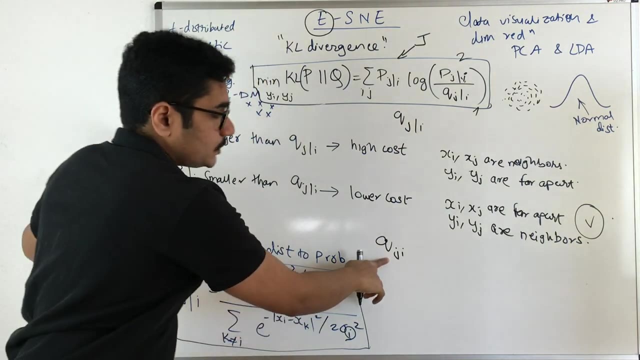 So we had that representation with Sigma removed. So we now apply a T distribution to this. So whenever we apply a T distribution to a symmetric function, it reduces to Q, say J, I. now this is no longer conditional probability, We take a joint probability here. 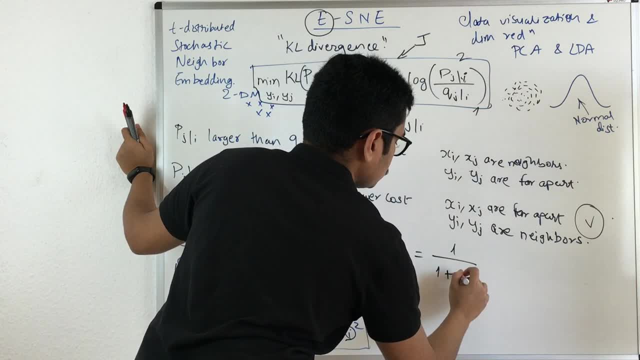 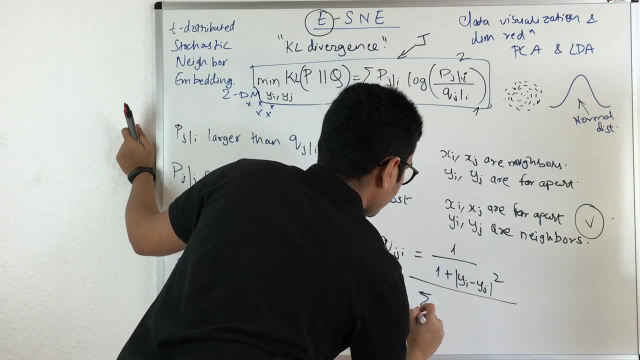 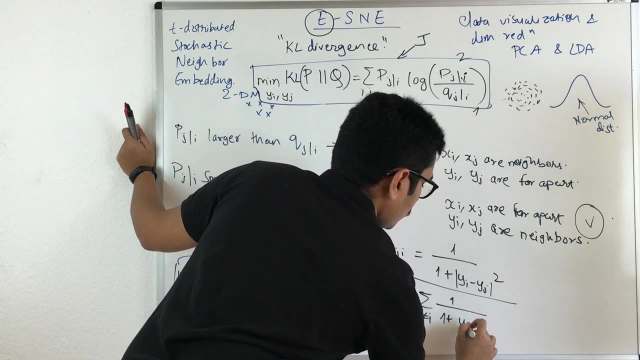 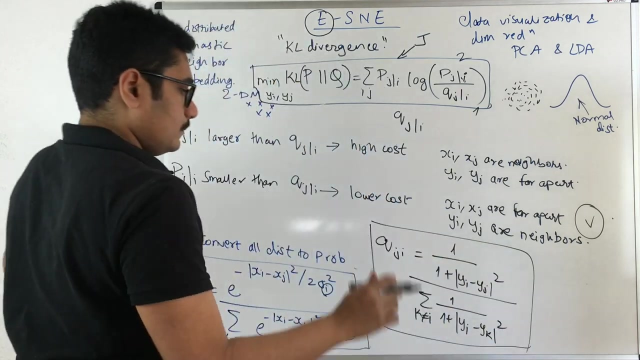 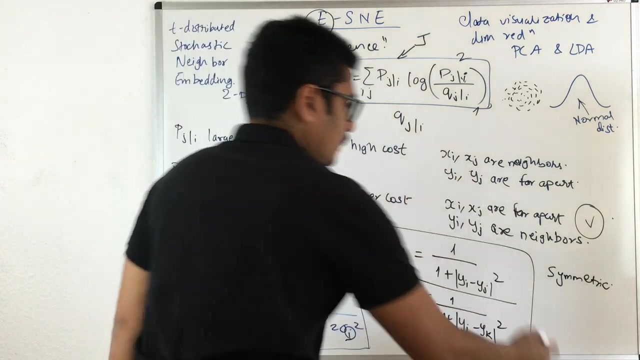 So this becomes 1 upon 1 plus YI minus YJ square upon Sigma times K, not equal to I, 1 upon 1 plus YI minus YK square. So this particular function is both symmetric. So first we convert it to symmetric and then we apply a T distribution. 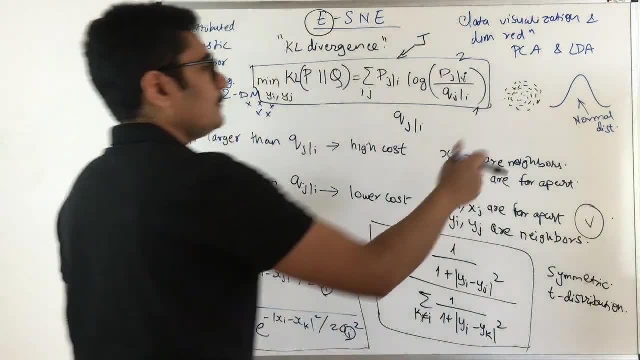 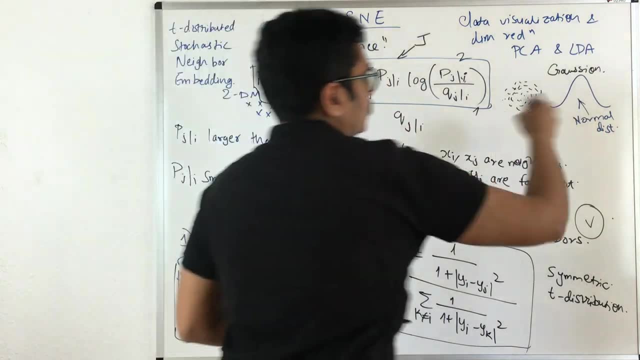 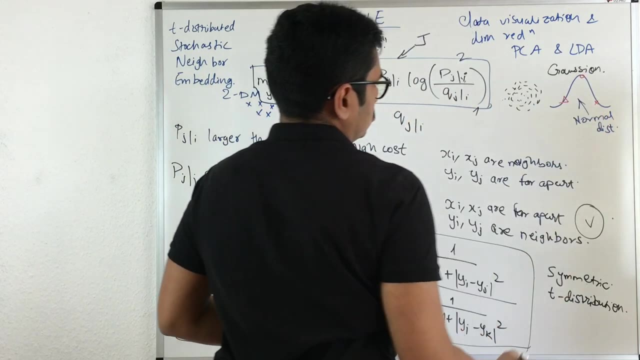 And why we mainly use T distribution is because, say, this is our original Gaussian or for normal distribution. So here what we say. for example, if you have any point, say like this, and if you have another point, say like this, and you have say another point like this, the probability of this point being closer to this distribution is very higher. 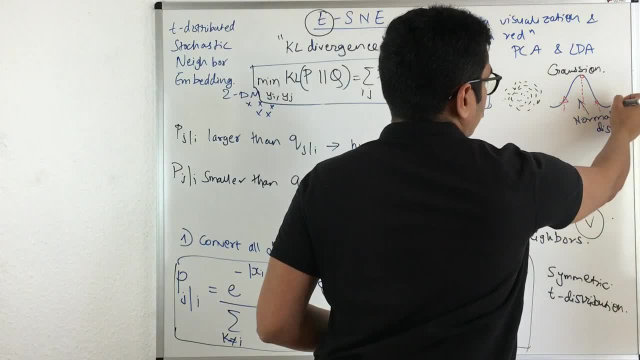 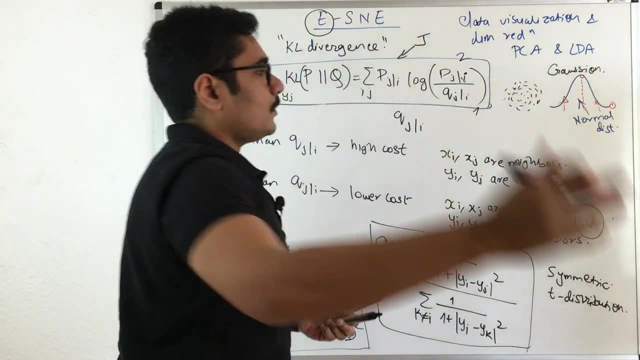 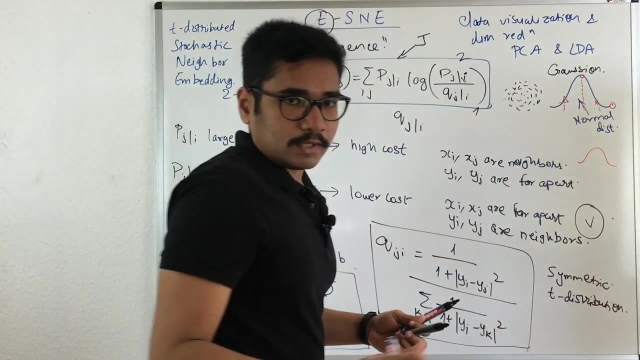 But for other points, say if you have any number of other points. So similarly, if you have a same point like this for the same distribution, It's just Away from your normal distribution. So it's essentially you have a curve like this, You don't have longer tails, but T distribution essentially gives you a visualization for longer tails. 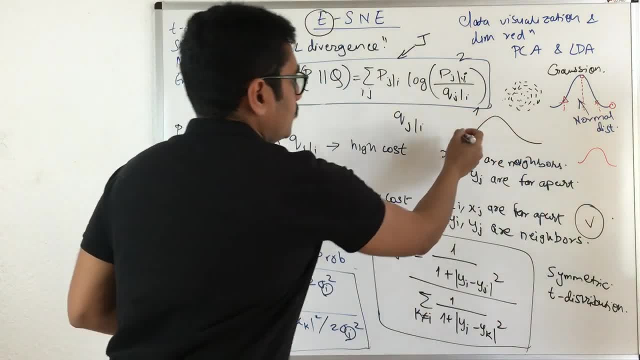 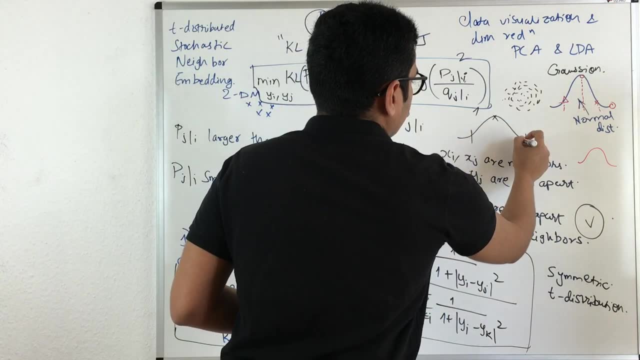 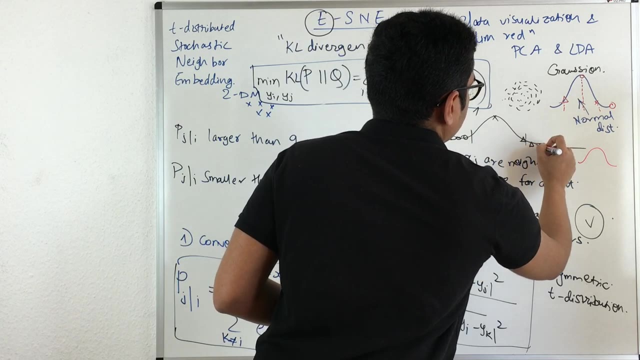 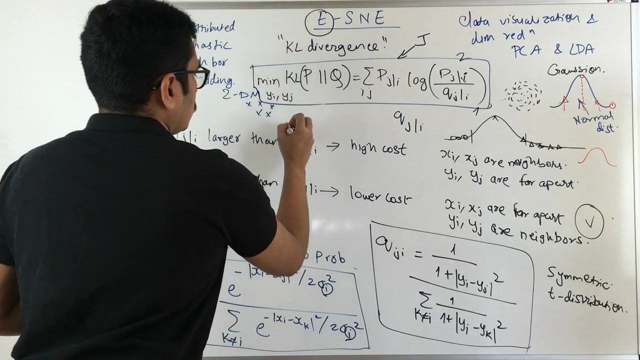 So you don't have a bulge at the center. instead you have longer tails. So this is nothing but your tail. So if anywhere you have points, say here, or if you have point here or here, It will just Make it its tail large, so that you can accompany this. and also whenever we saw that particular number line where we had different points in the original dimension. 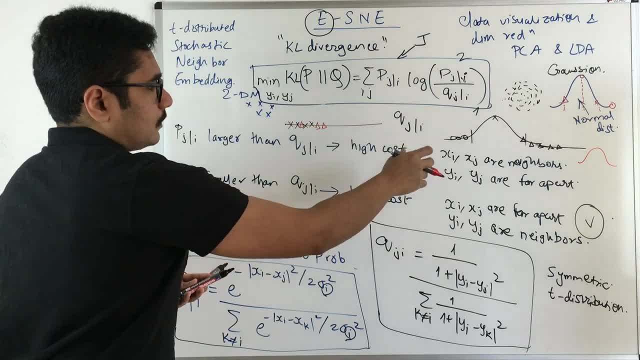 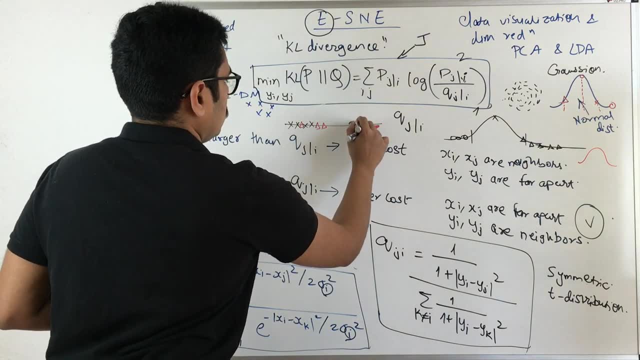 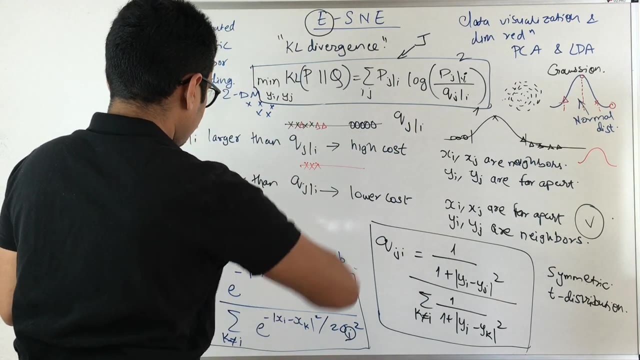 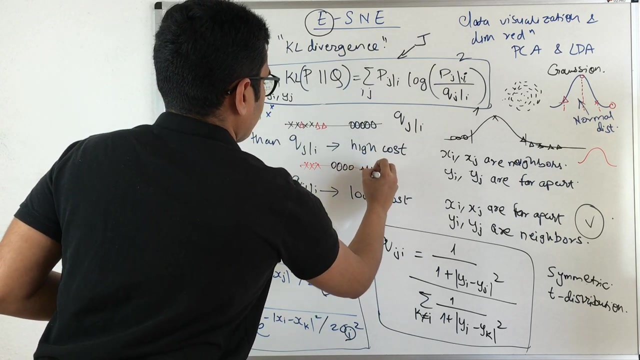 We had a mixture of these things. So now, since we have a T distribution here, what we can achieve is we can have a well separation of all these different points. So now our points are Like this: So now our original objective, that what we want is mainly achieved with the help of this distribution. 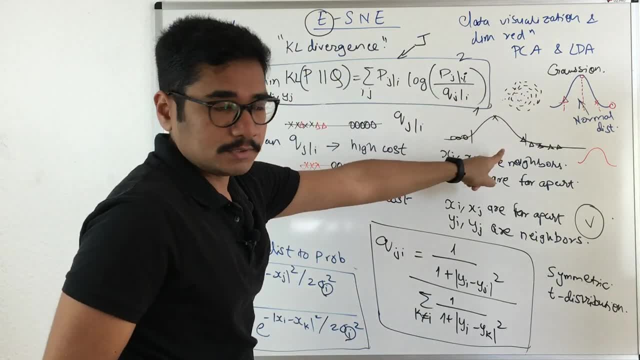 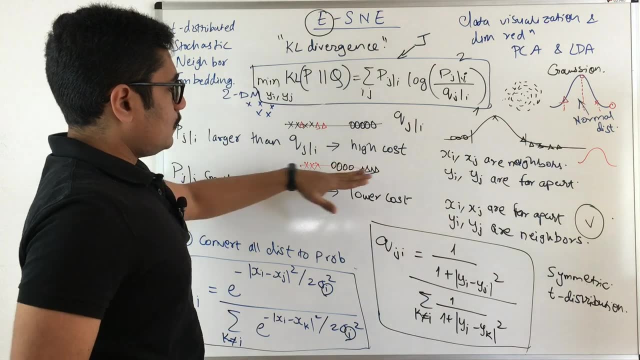 So in our Gaussian we got this, but when we use the distribution it has a longer tail so that it can separate each of the points towards its left or towards its right. We can have this distribution. So this is all about the t-SNE. 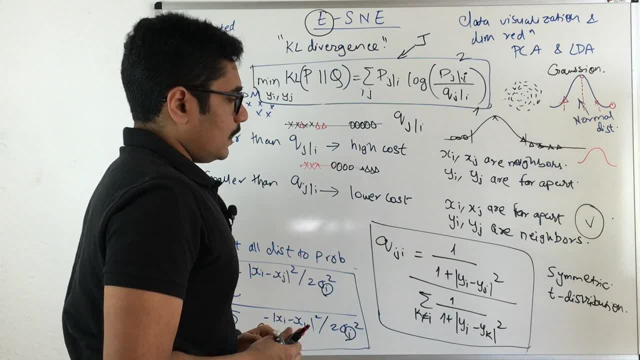 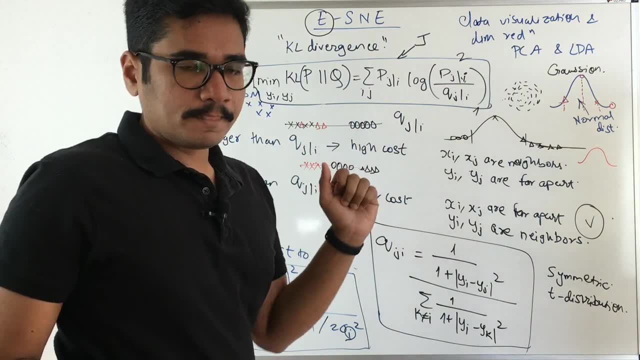 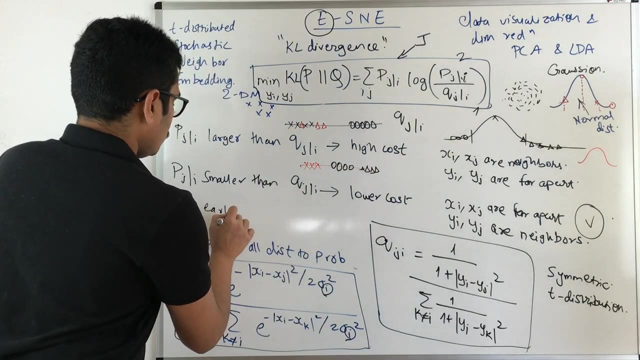 Now Just one reminder about t-SNE. In different papers, in different research paper, You can see there are different heuristics that can be applied to t-SNE. Now there is one heuristic by which this algorithm learns that is called as early exaggeration. 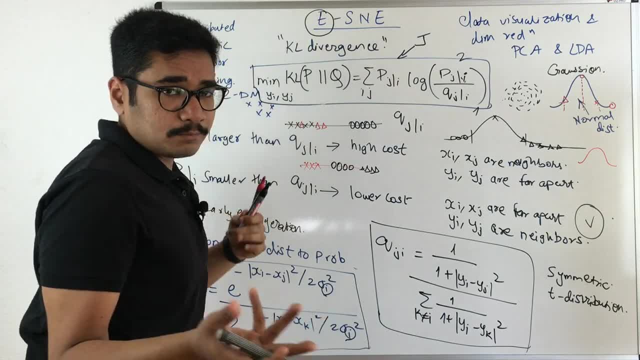 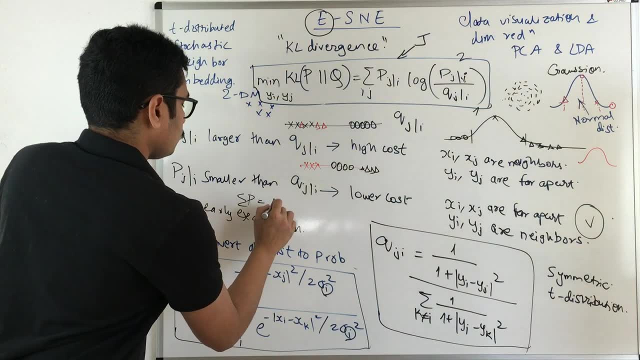 Now what early exaggeration means that if you have large number of data sets and if you have very few points, What it does is it will just sum up the probability values as 4. so that is just a brute force value. you add up to this. 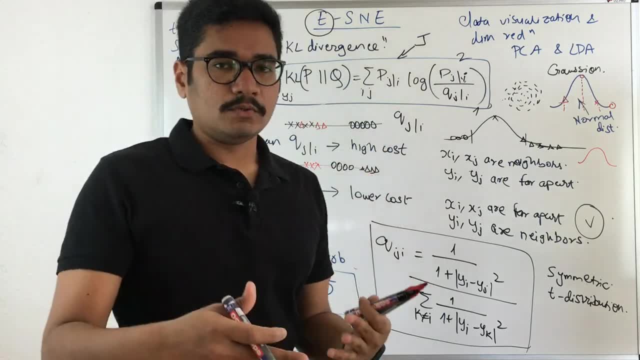 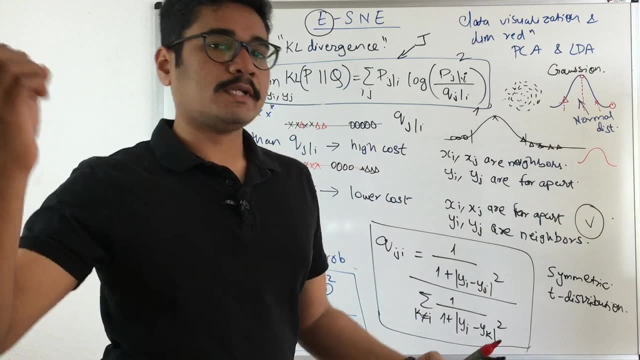 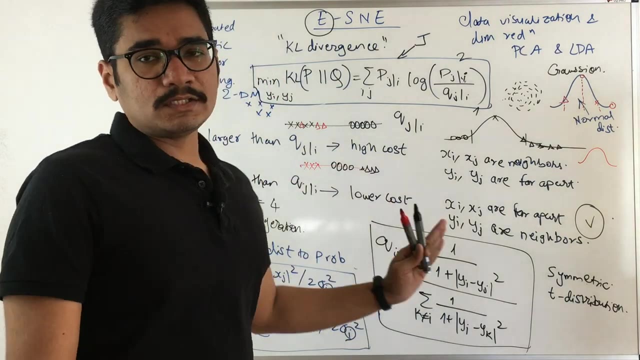 So what essentially does is, whichever points are very close or whichever needs to be considered very first, it will consider those points, and all the important other points, which are most of the representative of your original distribution, are just kept aside. So that's not a very good approach for this, and so this essentially has a drawback when dealing with larger data sets. 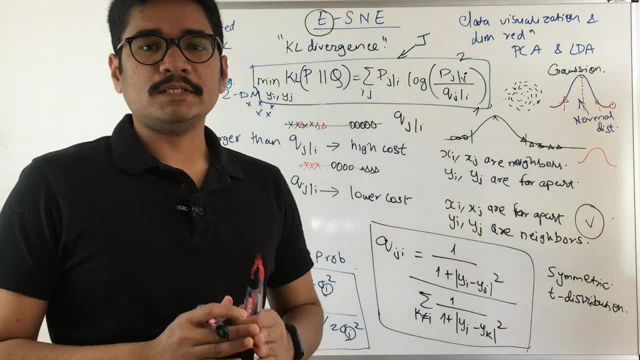 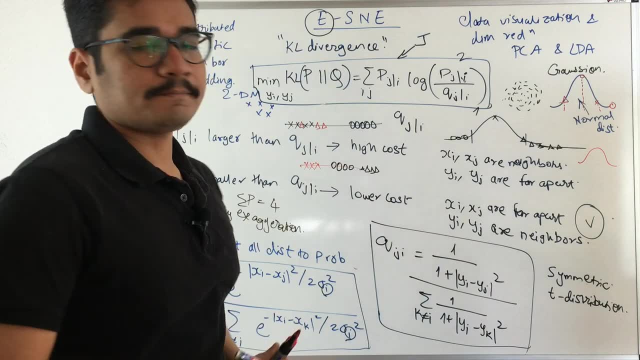 So that is one important drawback of the t-SNE, and you have both visualization and dimensional detection technique going hand-on-hand with this technique. So well, that was all regarding the t-SNE approach in machine learning, So hope you guys enjoyed this video.